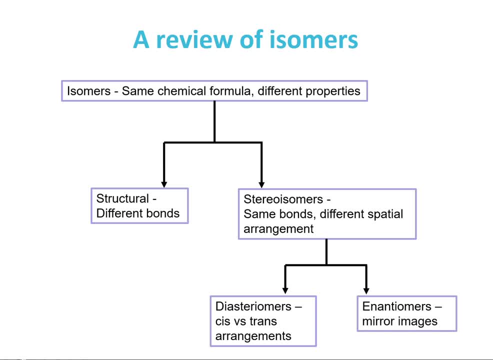 terminology, An isomer is a compound that has this: they have the same chemical formula but different properties, and from there you can branch off to talk about structural isomers which have different bonds. We're not talking about those. We're talking about stereoisomers, which 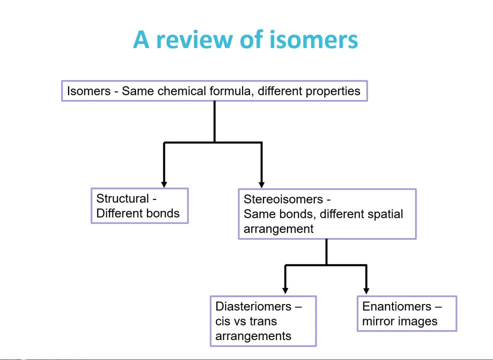 have the same bonds but different spatial arrangements and within that category, you can have diastereomers- where you're talking about cis- versus trans arrangements, or enantiomers, and those are the mirror images. That's what we're talking about today when we talk about amino acids, enantiomers. So just a. 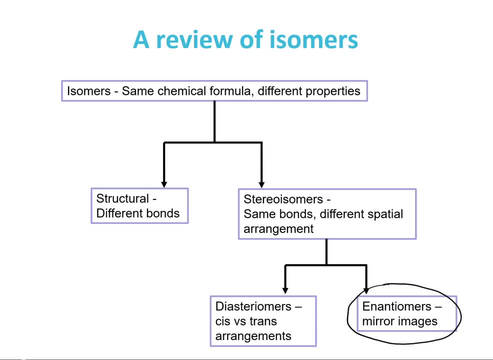 heads up. if you don't remember that, from general chemistry slash organic chemistry, you may want to go back and review that. We're not going to be too heavy in labeling things as diastereomers versus enantiomers or anything like that, but you want to make sure that you understand what an 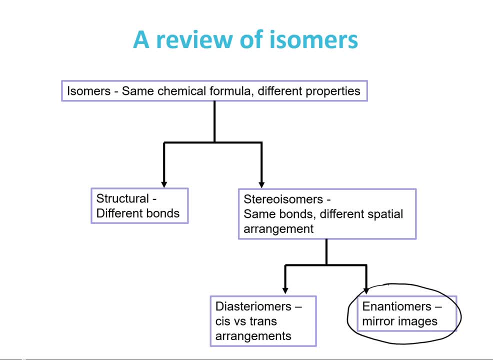 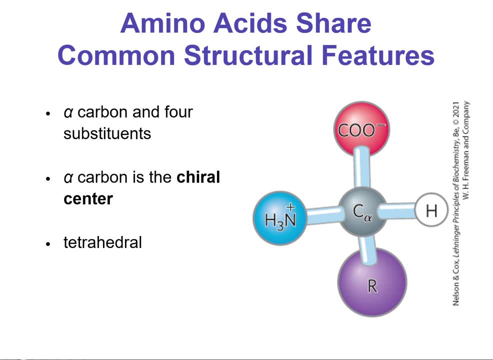 enantiomer is and what that means in terms of amino acids. So this is the generic structure for an enantiomer: There's an alpha carbon at the center and that alpha carbon is the chiral center. All amino acids, except for glycine, have a chiral carbon at the 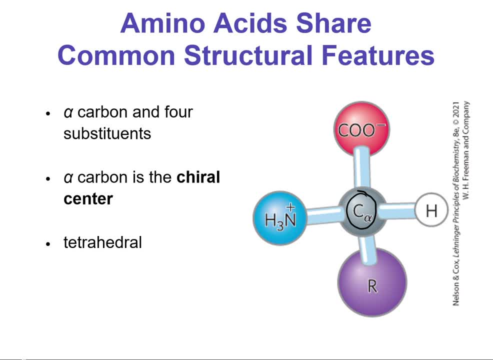 center, The shape is tetrahedral, and they all have this amino group here And this carboxylic acid, There's a hydrogen and then there's this R group, which is different depending on the side chain. The side chain is what gives each 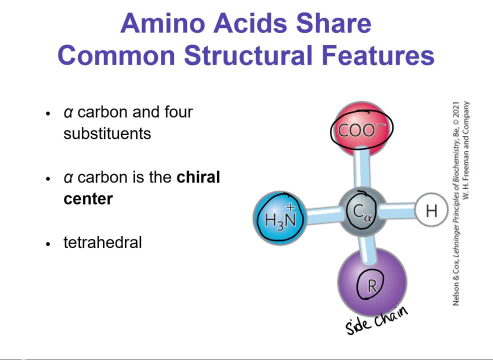 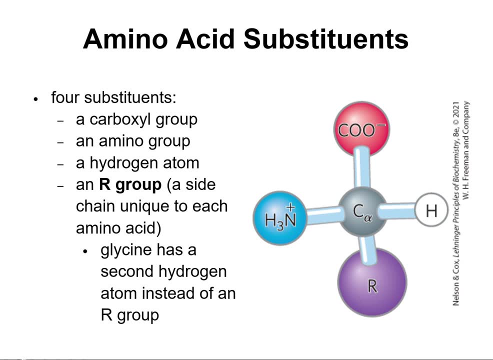 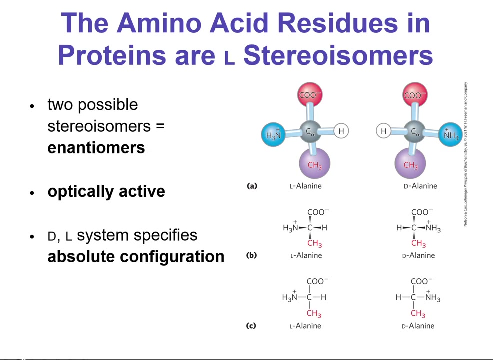 amino acid its own little flare. So we just went over all of these: The carboxyl group, amino group hydrogen, and then the R group, which is the side chain. there are actually two possible stereoisomers for amino acids and they are enantiomers. 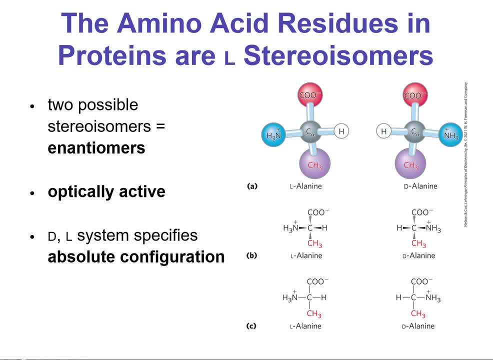 which means that they are a mirror image of each other. so if you were to have a mirror right here, what you would reflect is if you're looking, if you have the L alanine, let's say looking in the mirror, what you would see is D alanine. 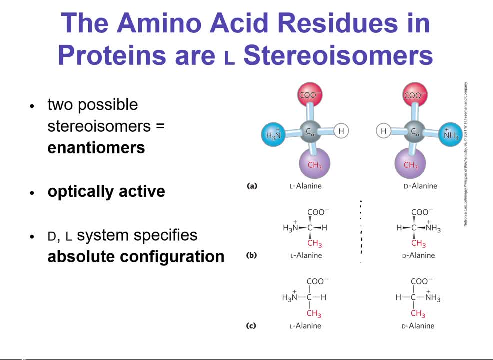 and this matters because the spatial arrangement means different things in terms of binding, optically active. that just means that if you had two separate mixtures, one of L alanine, pure L alanine, the other one of pure D alanine, let's say, since we have alanine on the slide here, then you would see different. you'd see. 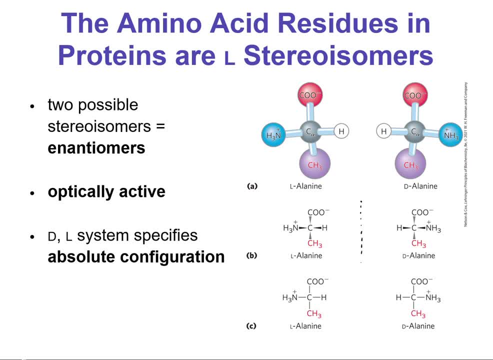 differences in terms of how the those two compounds interact with light. so all this means is that these enantiomers interact with light differently, and you can detect that, not going heavy into that either. I just want you to know that that's what optically active light is, and you can detect that, not going heavy into that either. I just want you to know that that's what optically active light is. 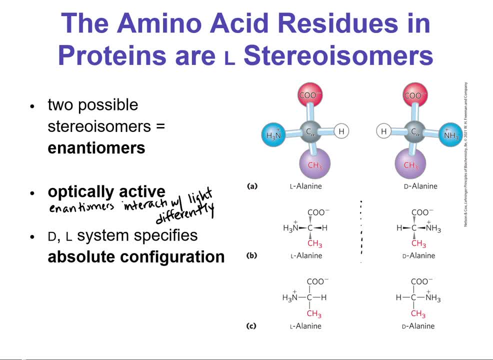 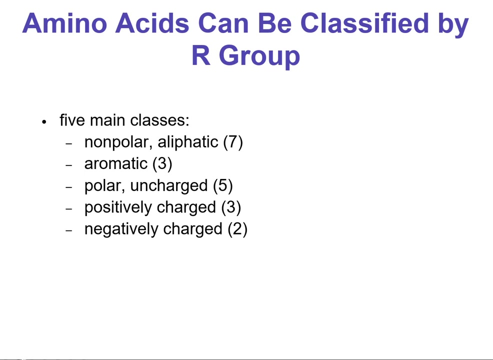 means, when you're looking at amino acids, there's the D and the L, and that tells you what configuration amino acids you're looking at. for our purposes, we're focused on the L amino acids, because that's what you see in proteins. there are five main classes of amino acids: nonpolar, aliphatic, aromatic, polar. 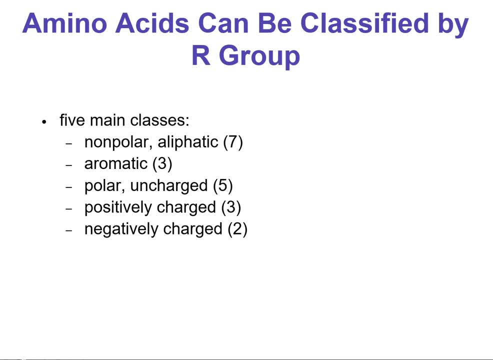 uncharged. positively charged, negatively charged. you may be used to seeing fewer classes. sometimes these two groups are lumped together to just say hydrophobic and these groups are lumped together to just say charged. but we're going to have a little bit more detail in this class. let's start. 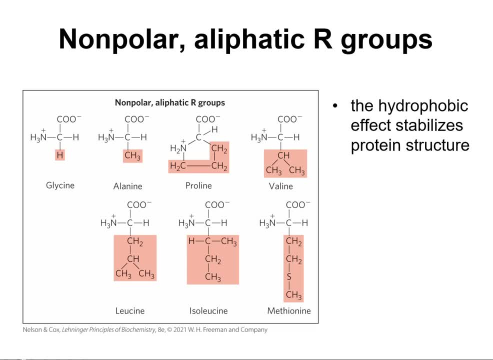 with the nonpolar aliphatic groups. right? so, like we said before, all amino acids have the same amino group- carboxyl group and hydrogen- but what's highlighted in this coral color is the R group, and that's what gives them their specific properties. aliphatic simply means like a carbon chain will be a little more. 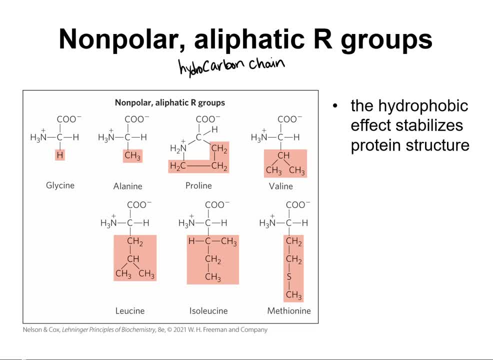 specific hydrocarbon chain. now there's one exception here. there's a sulfur in this methionine, but it's still largely it's an aliphatic group. okay, so all of these are nonpolar in nature and the hydrophobic effect that we talked about in chapter two. 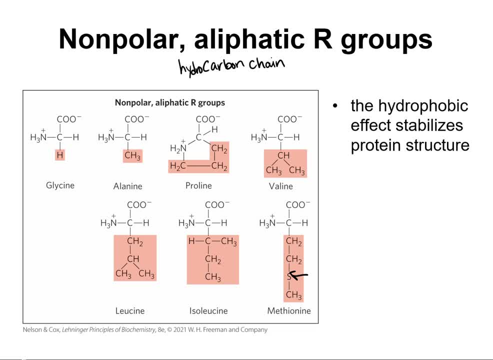 these amino acids help stabilize protein structure. through that hydrophobic effect, they will cluster together and become stable and sequester themselves away from water. you will need to memorize your amino acids for this class. you'll need to be able to recognize them and draw them. 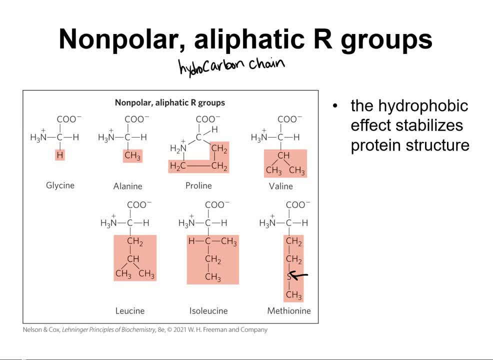 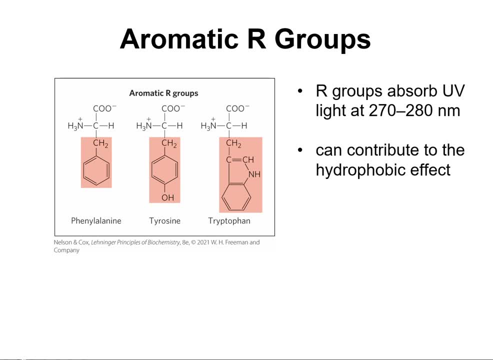 you'll also need to be able to draw short peptides as well. we'll get to that in a second. the next group is aromatic R groups. so these are the ones that have some kind of they've got- double bonds. you see this benzene structure as a 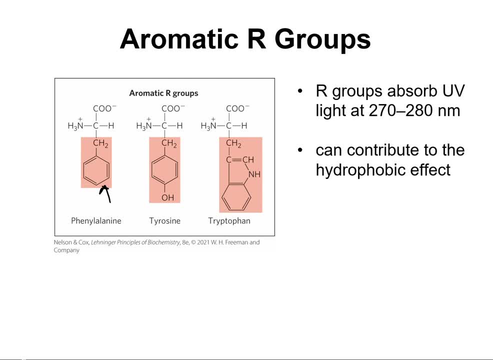 part of all of them. they absorb light somewhere in the 270 to 280 nanometer range And when you're looking for protein concentrations and you're looking at that particular wavelength of light- around 280,, you're looking at these amino acids. Now, all proteins don't have a high concentration of phenylalanine, tyrosine or tryptophan. 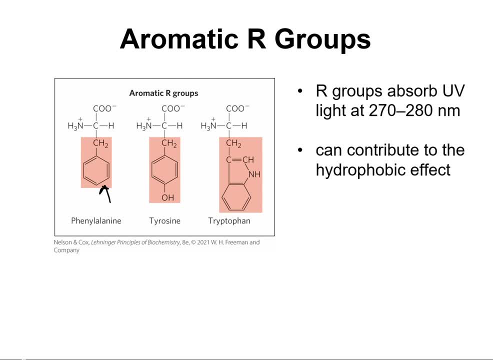 So if they had kind of reduced numbers of these particular residues, you're not really going to see it that well. So that's just if you're in the lab tip. These groups can also contribute to the hydrophobic effect, just like the nonpolar aliphatic groups. 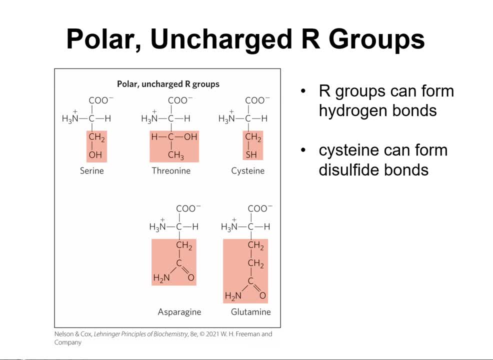 Then we've got the polar uncharged R groups So they can form hydrogen bonds. Cysteine is special because it can form disulfide bonds, So it will make bonds with other cysteine residues And form these disulfide bonds which you may also see termed disulfide bridges. 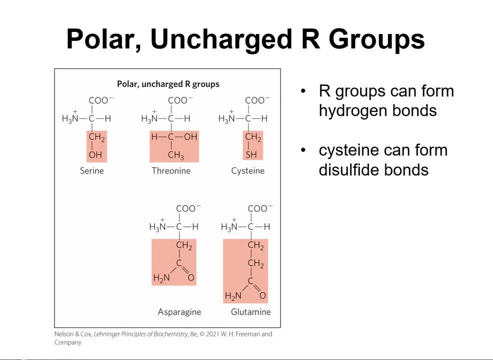 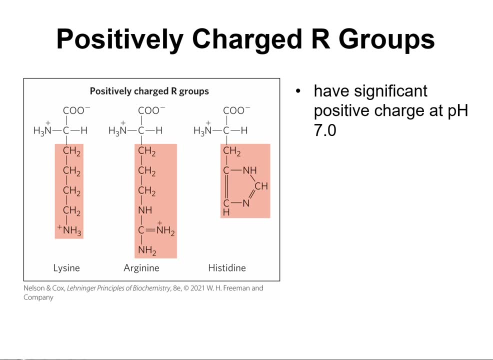 And those are also very important for protein structure. We've got positively charged R groups. They have a significant positive charge at a pH of 7. And remember from chapter 2, pH 7-ish is pretty biologically relevant, So the charge around this pH is definitely relevant. 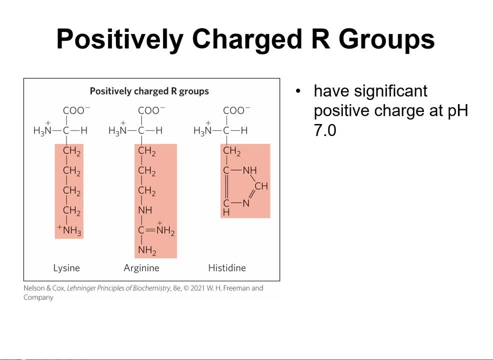 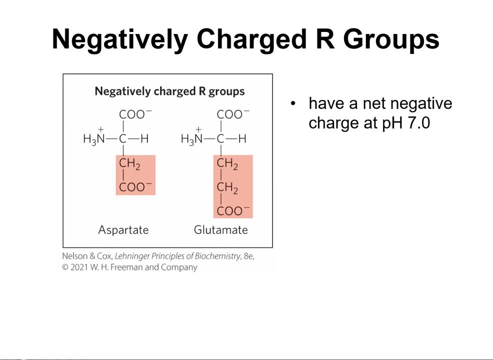 It's also relevant to protein structure and function. Then we've got the negatively charged R groups And they have a net negative charge at pH 7.. Again, you'll need to know these. So make sure that you recognize the structures and that you know the names. 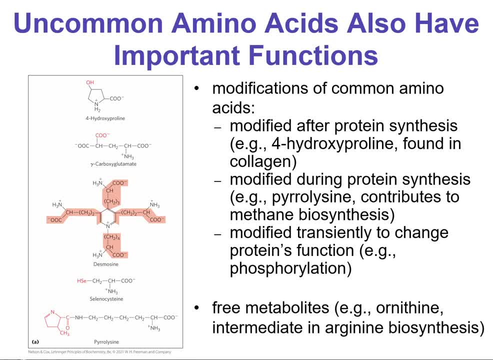 There's also some uncommon amino acids that have important functions. You don't need to memorize this, This is just for your own edification. So some common ones are: 4-hydroxyproline, And that is a modification that happens after a protein is synthesized. 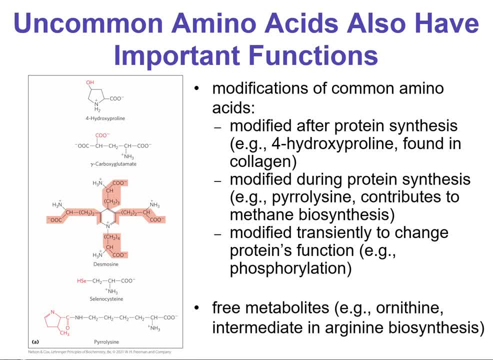 And it's found in collagen. Then sometimes you have modifications that occur during protein synthesis, such as pyrolysin, Another one we've got modified transiently to change a protein's function, like phosphorylation. We're going to talk a lot about those, especially when it comes to metabolism. 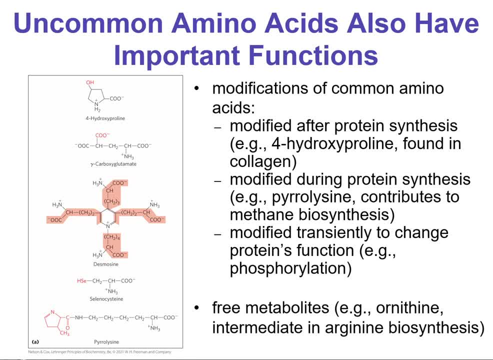 And then we have some free metabolites like ornithine. It's an intermediate in arginine biosynthesis. Sometimes intermediates can act as part of feedback mechanisms to control metabolic processes. So all of these are uncommon amino acids Examples that actually have pretty big roles. 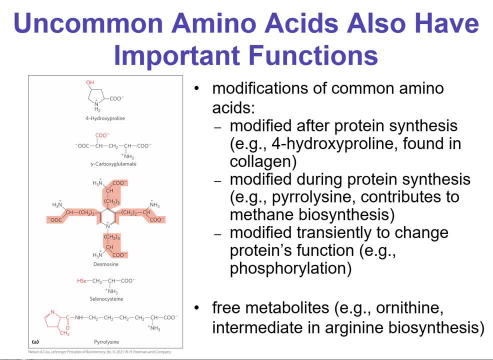 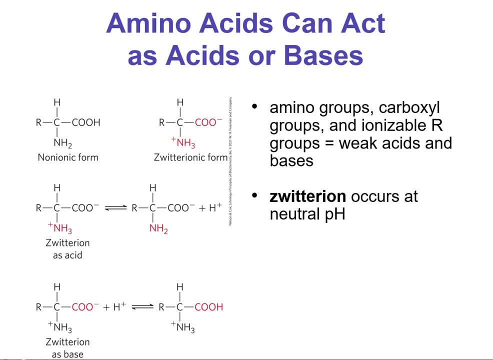 Again, you don't need to memorize this. This is just for your knowledge. Amino acids can act as acids or bases. So if you're a little bit shaky on chapter two with how weak acids and weak bases, you know we talked about equilibrium and pKa's and things like that. 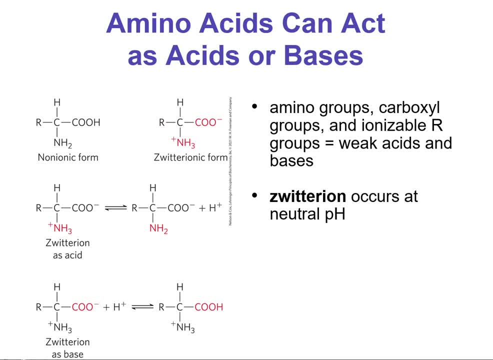 You'll definitely want to shore yourself up on that And then revisit the amino acids. All amino acids have a non-ionic form- I'm going to break up my highlighter here- And in this non-ionic form, that means that there's no charge. 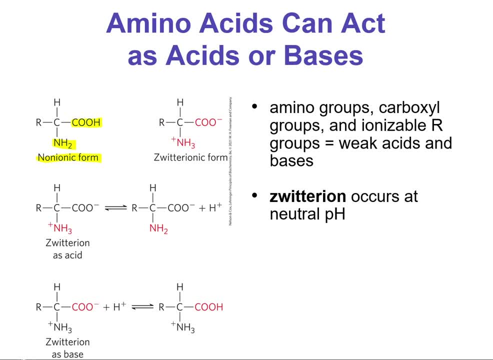 So NH2COOH: no charge there. The zwitterion form: we've gained a hydrogen here and we've lost a hydrogen here. The zwitterion occurs around neutral pH And what that means is that this form has a net zero charge. 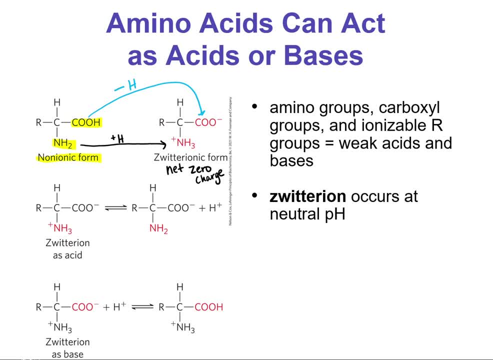 So that's the zwitterion net zero charge. Zwitterions can act as an acid or a base. If it's acting as an acid, it's going to lose a hydrogen or donate a hydrogen. So I'm just highlighting here: 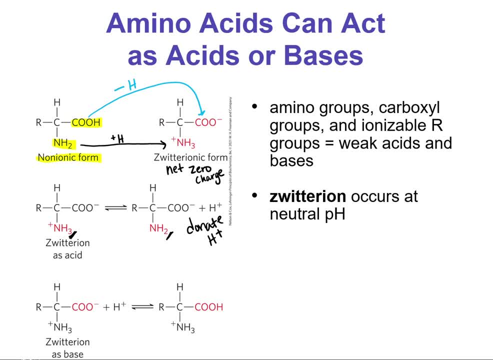 We go from that NH3 to NH2. So we're donating a hydrogen. Zwitterions can act as a base by picking up an extra hydrogen. So in thisici power here, the rectangle over here is the practically second- atom. So 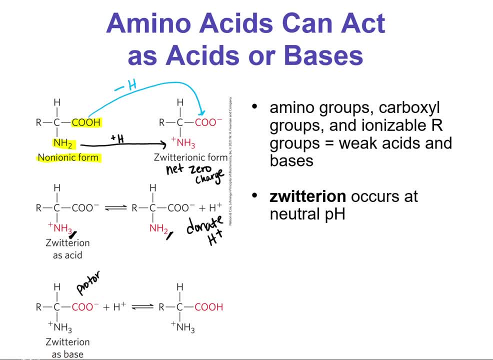 every eigenvector could be a hydrogen. We should write that on the other side. So this acts as a proton acceptor And we go from a negative charge here to no charge, And we go from a negative charge here to no charge. 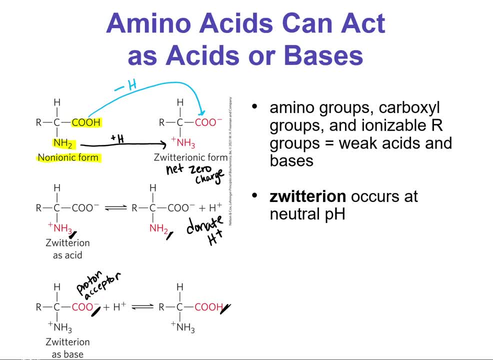 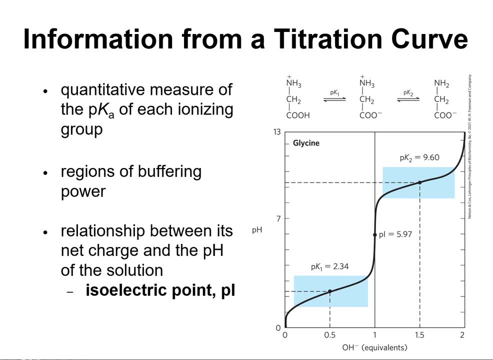 Here. here's another simple result. Here's what's the quality of the base And we should. So the zwitter ions are very important When we're looking at a titration curve like the ones we talked about in chapter 2, we 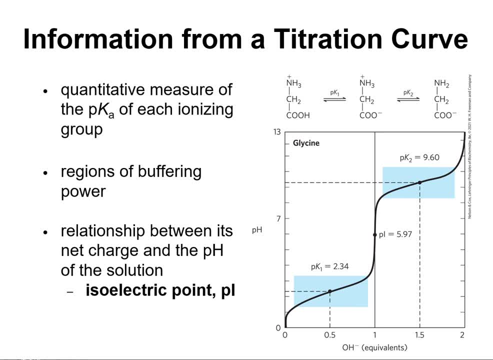 can get a lot of information. We can get the pKa of each ionizing group from an amino acid. So each amino acid has at least two ionizing groups: The amino group and the carboxyl group. Right now we're looking at glycine and its titration curve. 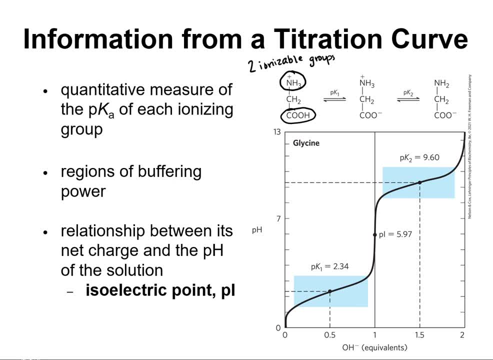 So we're going to look at glycine and its titration curve. Its R group is just another hydrogen, clearly not hydrolyzable. it is connected to a carbon. What this means is that, since you have two ionizable groups, there are two regions of. 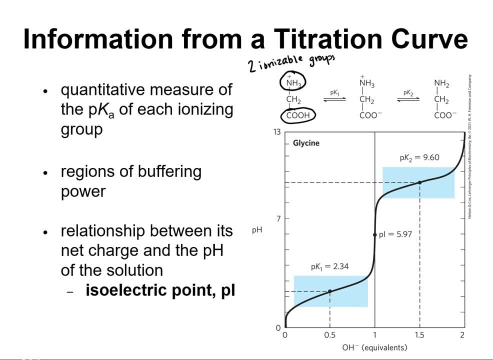 buffering power. So these blue rectangles show the two different buffering zones that glycine has because of these two ionizable groups. You'll notice this Pi, which we haven't introduced Pi yet. Pi is the isoelectric point. The isoelectric point is the point where you have the ion, the zwitter ion, with the net. 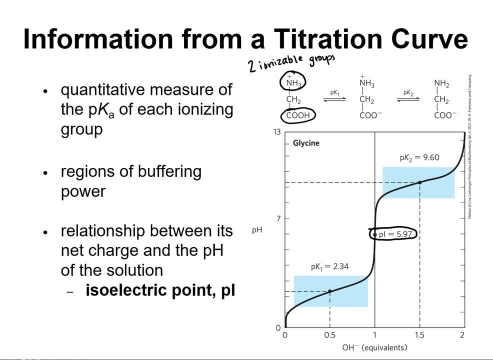 zero charge. Okay, So if we look at this and try to figure out which species of glycine was present at very low pH, You're going to have this form here At about seven. so our Pi is 5.97.. 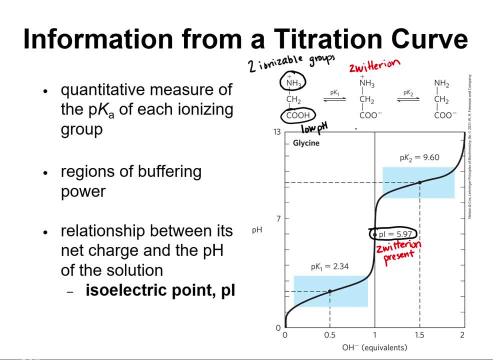 So somewhere around neutral pH you have that zwitter ion And then at high pH Or basic solution, you're going to have this last form. We're going to walk through this for different types of amino acids in class. I'll show you a couple more examples. 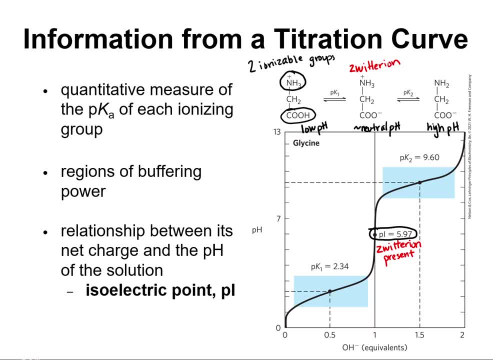 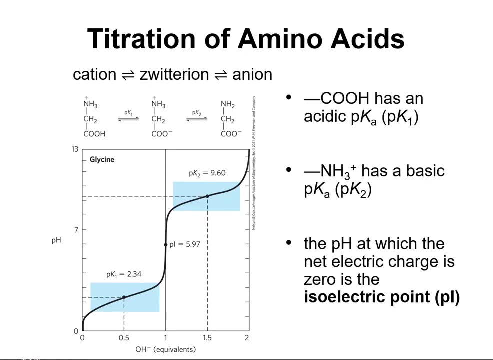 But understanding a titration curve and which species of amino acid is present is definitely something you'll need to do for this class. We're not finished talking about titration curves, but I want to give you the heads up now. So, in general, when you're looking at only two, 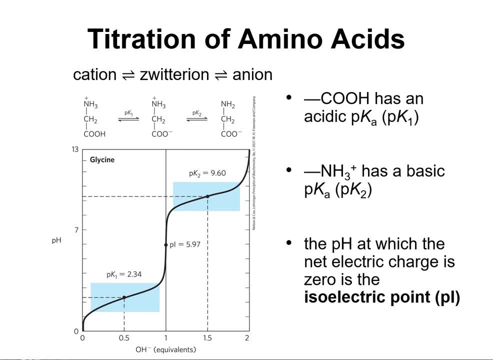 Ionizable groups, like with glycine, you start with the cation, which is something that's positively charged, Zwitter, ion, zero charge- and then anion, which is something that's negatively charged. Make sure that you understand this. We'll talk a little bit more about that isoelectric point. 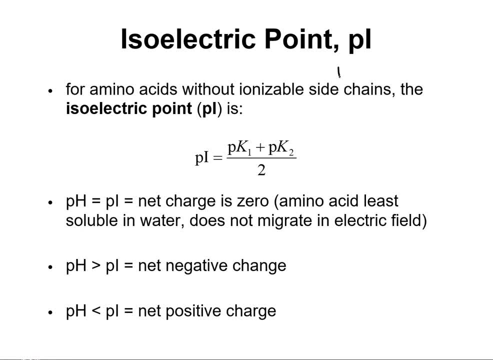 If you don't have an ionizable side chain- remember that our group- Then you can calculate the isoelectric point by taking the average of PK 1 and PK 2 and PK 1 and PK 2. it's another way of saying PK a, 1 and. 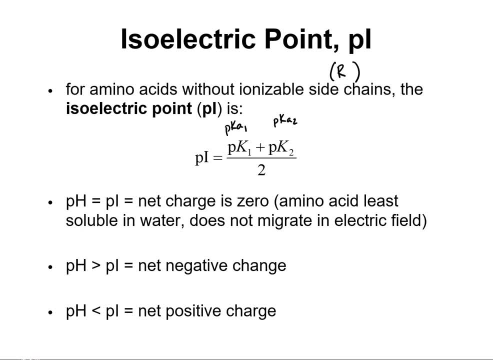 PK a 2 same thing. When you have pH that's equal to the PI, the number of points that are equal to the pI Net charge is zero. Your amino acid is not really going to be that soluble in water and it doesn't migrate in an electric field. It's got no charge. 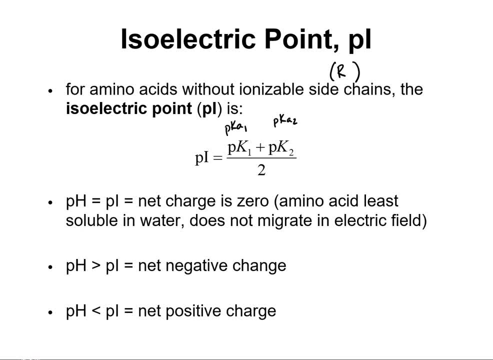 When the pH is greater than the pI, you're going to have a net negative charge, And when the pH is less than the pI, it's going to be a net positive charge. These are definitely things you should know, Because I can ask you a question about. 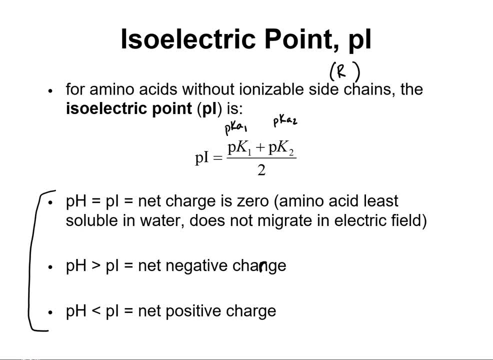 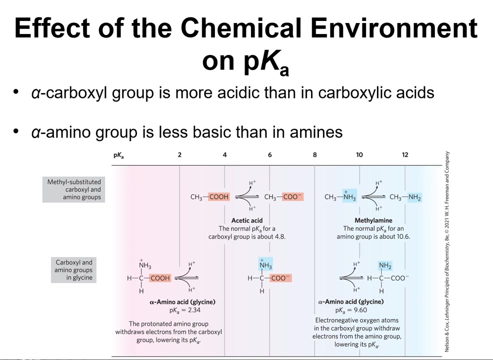 different amino acids, maybe that don't have ionizable side chains, so the nonpolar ones. and ask you, at pH X, What do you expect This amino acid to be? you know, is it positively charged, negatively charged, zero charge? So The pKa's for the carboxyl group and the amino group on an amino acid are: 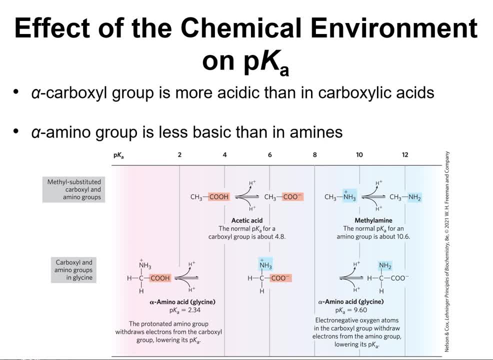 different from a carboxyl group on its own and amino groups on their own. The normal pKa for a carboxyl group is about 4.8, but It's lowered in this case because the amino group Withdraws electrons from the carboxyl group and that lowers its pKa. 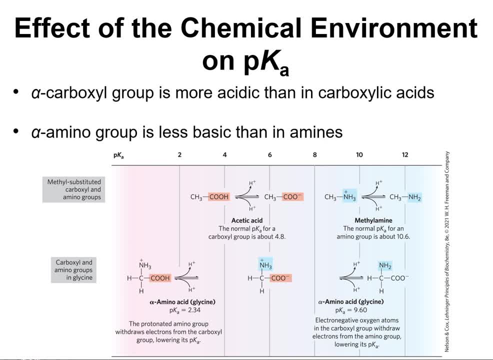 on the flip side, the amino group in amino acids Actually has a lower pKa as well because of the carboxyl group. so Normally the pKa for an amino group is about 10.6. So because these two groups are in close proximity, they affect each other's pKa. 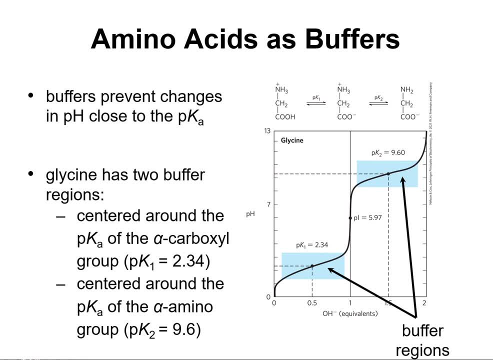 Since amino acids have these ionizable groups, they can act as buffers. We've got two buffering regions. The closer you are to a pKa, the better the buffer you have. If I gave you a titration curve, you should be able to tell me where the buffering regions are and 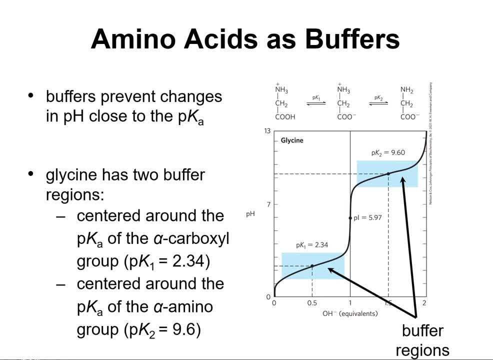 And what pH. you wouldn't want to have a buffer, so in this case You would not want to have. If you're trying to make a buffer at, say, seven, It's not going to work too well. Okay, so you should be able to look and see, okay. 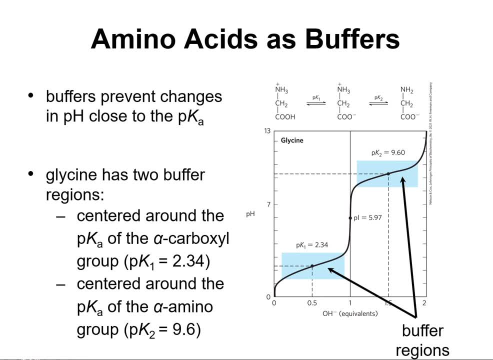 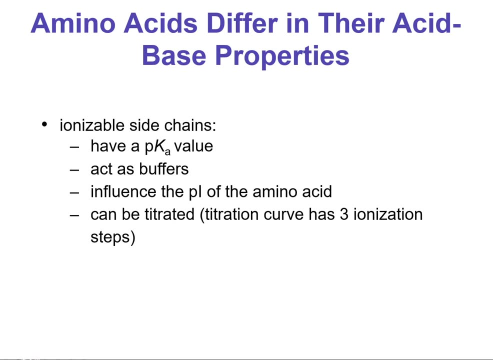 These are my buffering regions, These are the pHs I'd want to be close to about two and somewhere in the ballpark of ten. So remember those amino acids that have Ionizable side chains, like the negatively charged ones, positively charged ones. well, those side chains have a pKa value as well. so 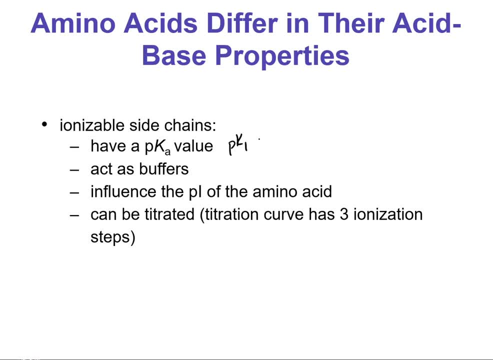 now, instead of just pKa 1 and pKa 2 we've got pKa 1, pKa 3, and They can act as buffers as well and they influence the pI of the amino acid. so if you have an ionized lil side chain, you can't just calculate the 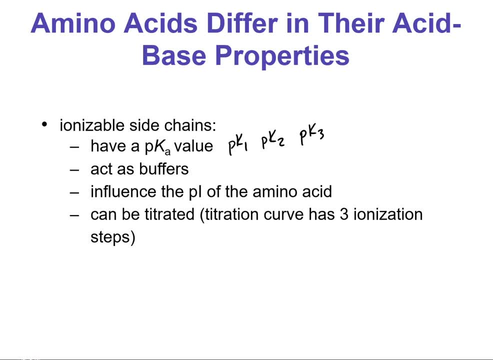 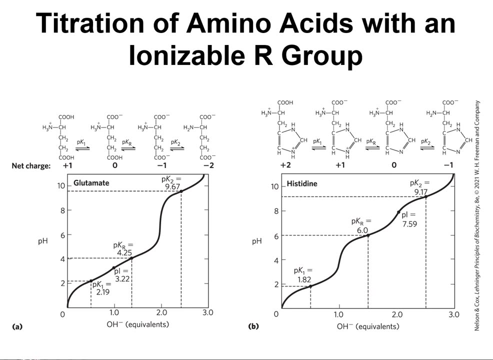 Pi, like you would with one that only has two ionizable groups. you can still do a titration, but you're going to have three ionization steps instead of two. So here are a couple of examples, And these look a little different than the glycine titration. 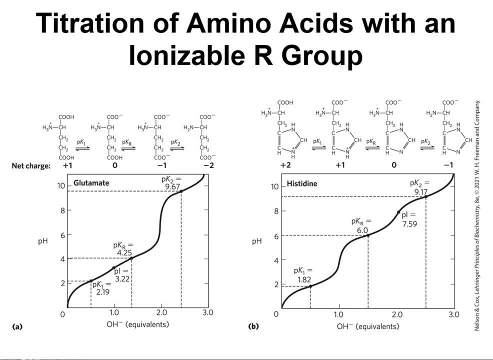 And you can see that you've got all these different PK. So you can have PK1,, PK2, PKR or 1,, 2,, 3.. So in your book you'll see PKR. I may use PK1,, 2, and 3.. 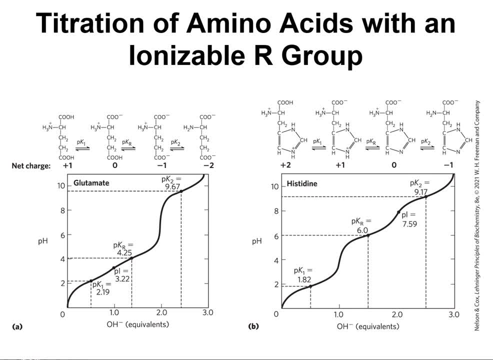 But understand it's the same thing. Looking at these structures and being able to tell the net charge is going to be key, Because that will tell you whether or not you're looking at one of the PKA's or if you're looking at the PI. 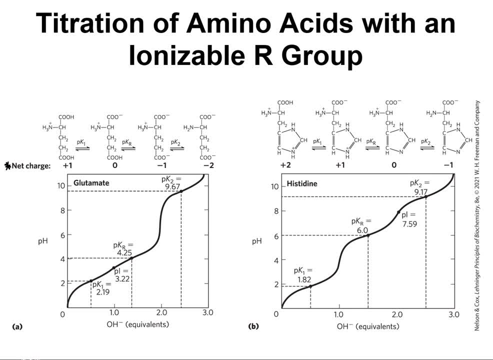 In the case of glutamate, your first value is PK1.. Then the next value that you get is your PI. when you're doing this, titration And knowing the different ionizable states of the amino acid will help you identify which points you're coming across as you're. 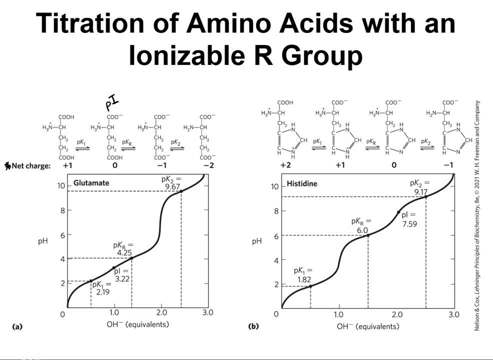 doing your titration. In the case of histidine, the order of events is PK1, PKR and then you're looking at the PI. That's where our zwitter ion is. So you want to take note of that charge. 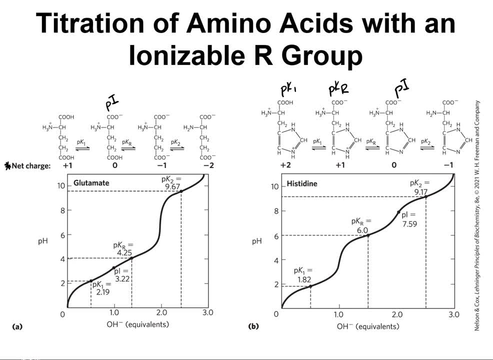 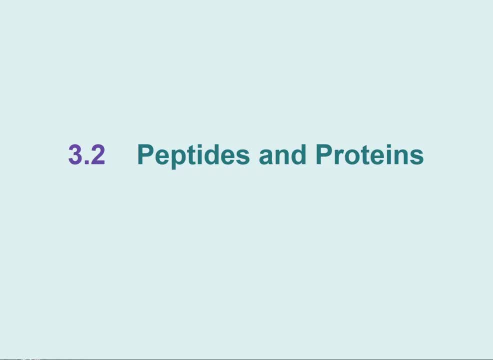 And again we're going to do this, We're going to do some practice and class to be able to identify these things: net charge, drawing the structures, that kind of thing. So that's amino acids. Now we're going to string them together to make peptides. 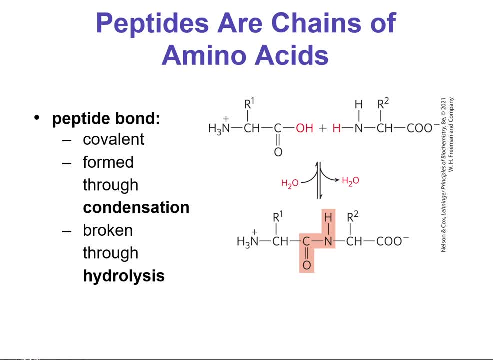 and proteins. Peptides are just chains of amino acids And they're formed by condensation of two amino acids. So you've got the OH from a carboxyl group on one amino acid and a hydrogen from the amino group on a second amino acid. 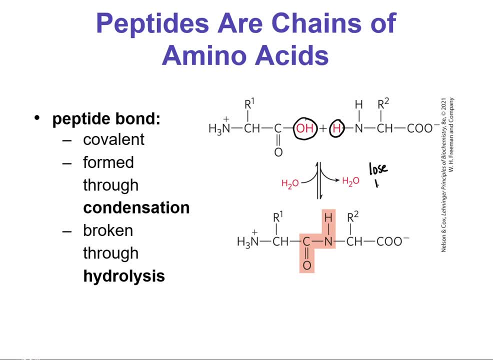 You lose a water and you form this peptide bond. This is an amide bond. You can also break these bonds through hydrolysis, So that is using water to cut this bond apart. So you can see here if you break these bonds. 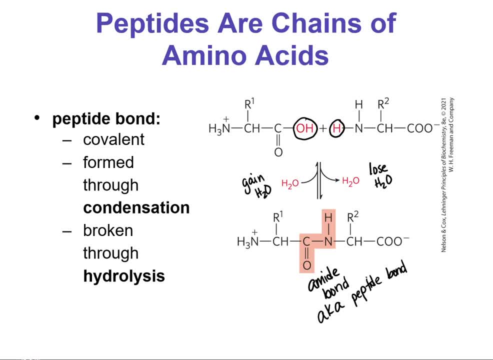 you're going to have hydrolysis. So you can see here, if you break these bonds, you're going to have hydrolysis. So you can see here, if you break these bonds, you're going to have hydrolysis. 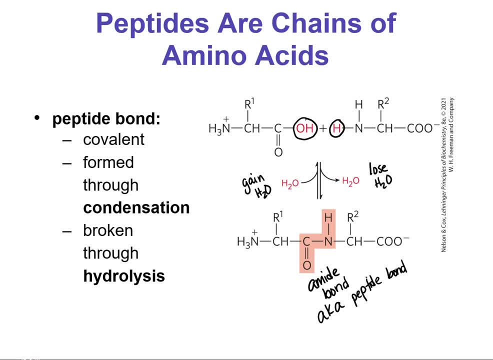 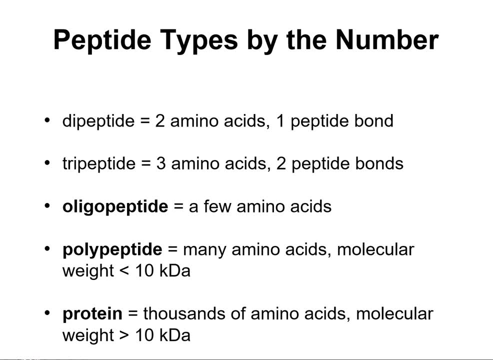 Not exactly as easy to do on the benchtop, but enzymes can do this quite easily. When we're talking about peptides, you can talk about them by the number. So a dipeptide is two amino acids, Tri means three, so that's three amino acids. 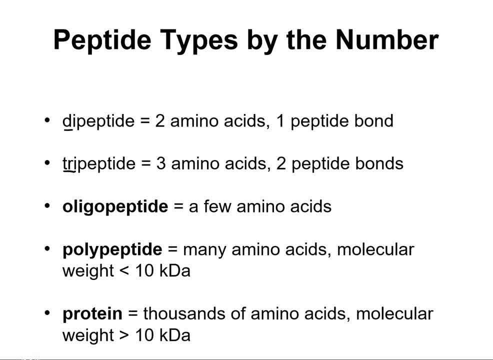 An oligopeptide. it's a short peptide. It's got a few amino acids. Polypeptide means that you've got something bigger more than 10 kilodaltons, And then proteins have thousands of amino acids, so much bigger than 10 kilodaltons. 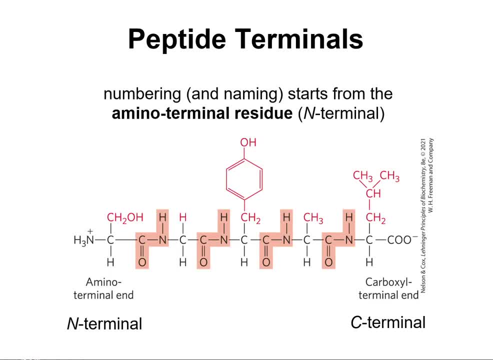 It's just a little terminology When it comes to numbering and naming. we're going to start with the amino acid. We're going to start with the amino terminal end. So notice this free amine here, this free amino group. That is the N terminal end. 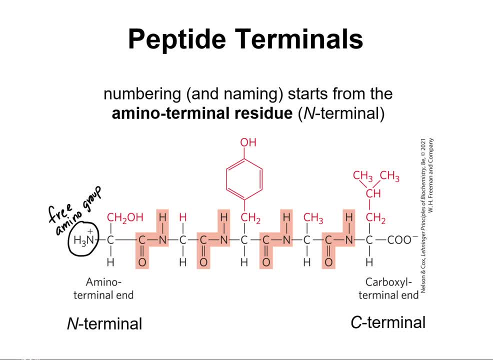 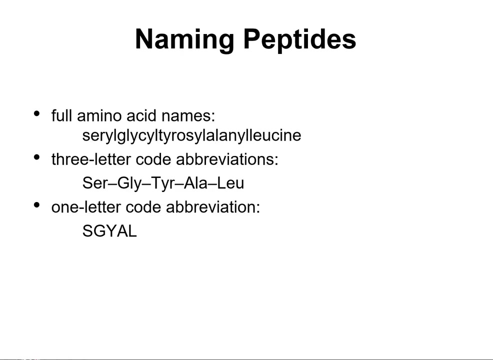 The amino terminal is what that N is short for. That is the beginning of the peptide. There are other residues, but your residue is just another way of saying amino acid. And then you have the carboxyl terminal end Thought I had a different slide for that. 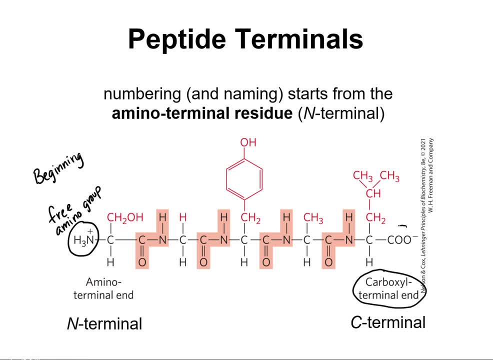 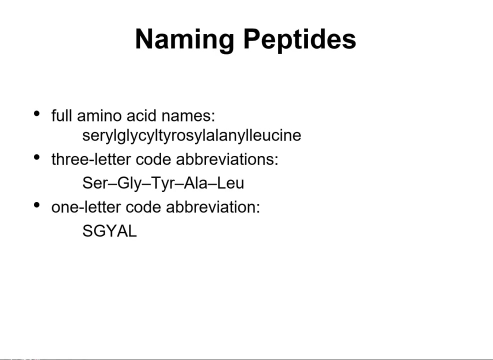 Apparently not. So. the carboxyl terminal end is here and that's just that. free carboxyl group. It's abbreviated C-terminal. When it comes to naming peptides, you can use the full amino acid names. We're not going to do that. 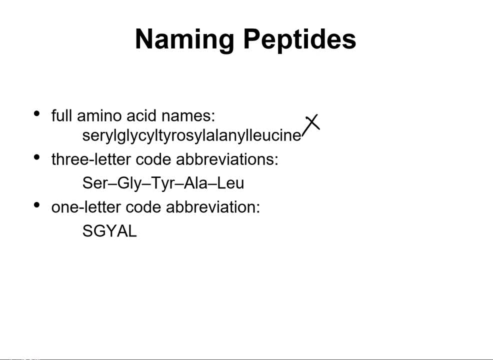 Ain't. nobody got time for that, But you will need to know the three-letter code abbreviations and the one-letter code abbreviations. So when you're memorizing the structures of the amino acids, you'll also need to know their three-letter code. 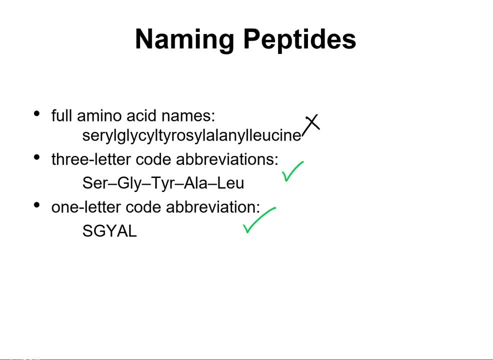 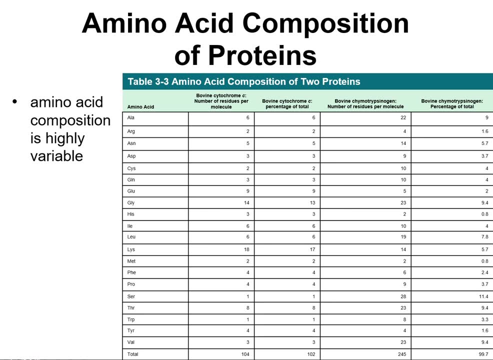 and the one-letter code. The amino acid composition of proteins is very highly variable, So this chart is just a partial looking at the amino acid. So this chart is just a partial looking at the amino acid. So this chart is just a partial looking at the amino acid. 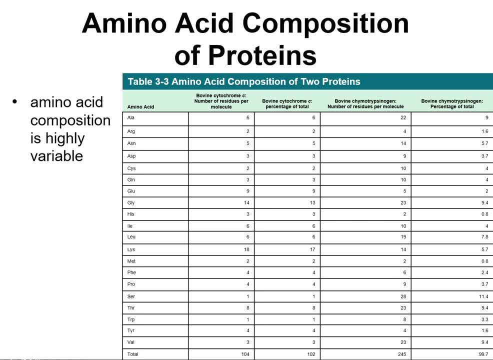 So this chart is just a partial. looking at cytochrome C. Cytochrome C is a part of the oxidative phosphorylation. It's all kind of linked in the mitochondria. We're going to talk about that when we talk about metabolism. 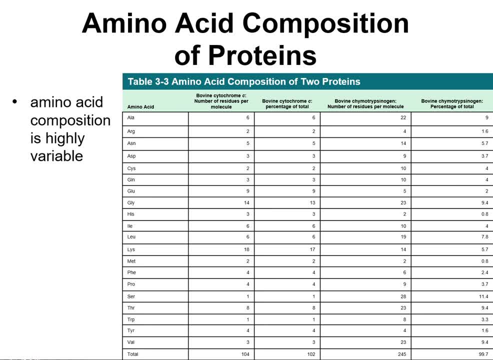 And you can find cytochrome C across different species. We also have chymotrypsogen in this table And we're looking at these two proteins and their composition. You know how many alanines, how many arginines? 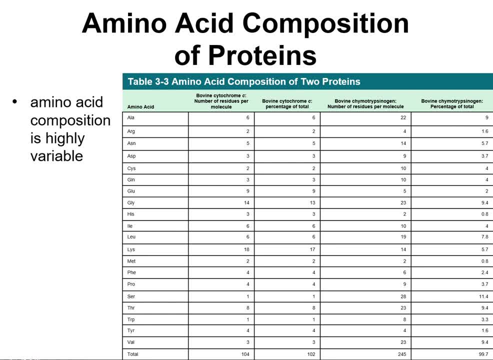 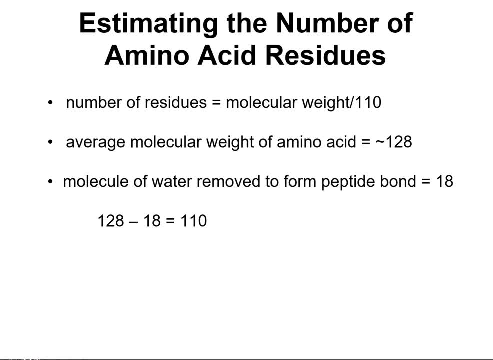 how many asparagines, all of that Wildly different, highly variable. That's all this slide says. You can estimate the number of amino acid residues, which I'm not really going to hold you back on that- hold you responsible for that- but it's just something that if you are interested in doing, 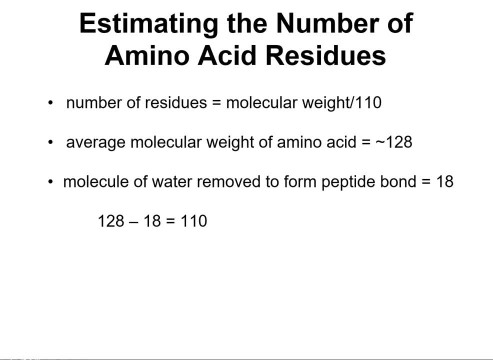 some kind of research. this is one of those tricks that you can use to get an idea of how many residues a protein has. So if the average molecular weight of an amino acid is approximately 128 daltons, and when you take two amino acids and condense them to form a peptide bond, 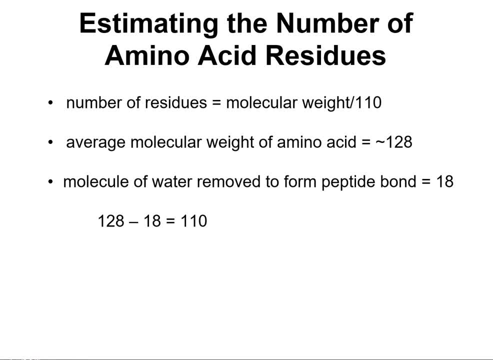 you're removing a water which is 18 daltons. So that means that on average you're going to have about 110 for each amino acid. So if you take the molecular weight of your whole protein divided by 110, that'll give you roughly the number of residues. 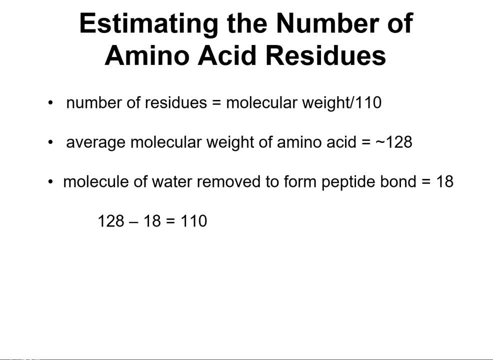 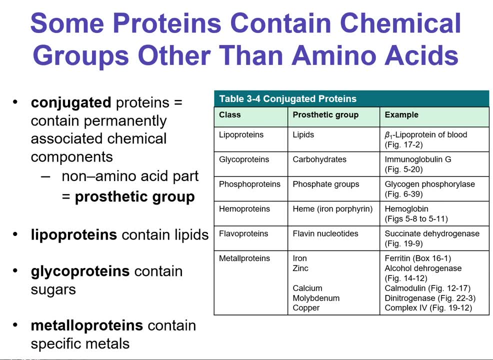 in that protein. Again, not going to hold you responsible for that. Now, all proteins are made of amino acids. Some proteins also have chemical groups aside from amino acids. So we've got conjugated proteins and they have a permanently associated chemical component. Emphasis on permanently. So the part that is the non-amino acid part is called a. 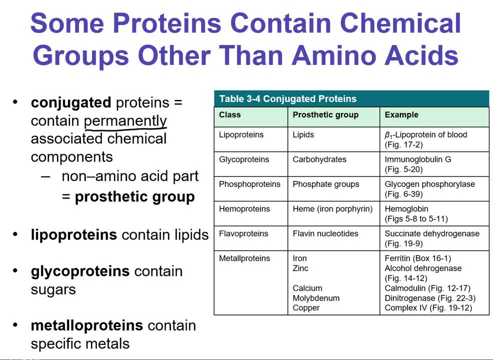 prosthetic group. So we've got plenty of examples. So there's lipoproteins that have lipids, Glycoproteins that have carbohydrates- You see that a lot in the immune system- Phosphoproteins: they have phosphate. 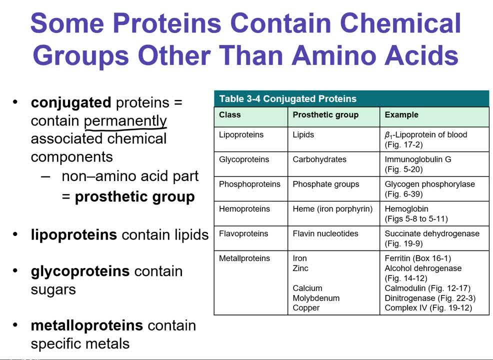 groups that are attached: Hemoproteins. so hemoglobin. we're going to talk about hemoglobin. It's got this iron porphyrin group, which is like it's an iron sulfur group. So it's got this iron porphyrin group, which is like it's an iron sulfur group. 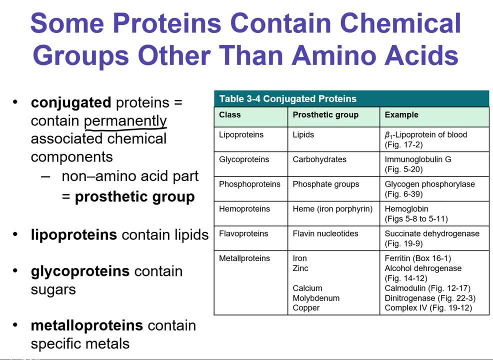 It's got this iron sulfur group. So lots of examples. Metalloproteins are very important and they require a metal for activity. So you see a lot of iron and zinc, magnesium- very, very popular in the cell- magnesium. So lots of examples of these types of proteins And that prosthetic group is 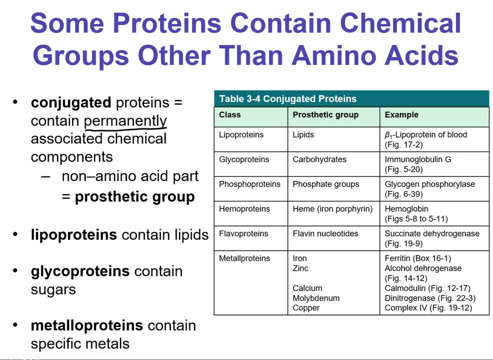 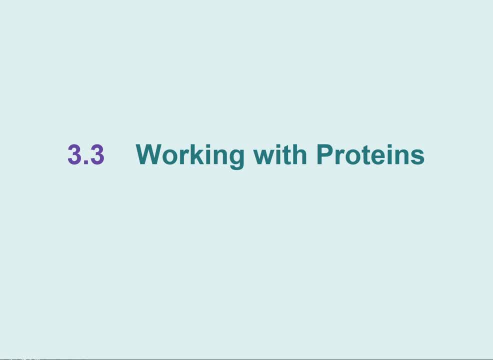 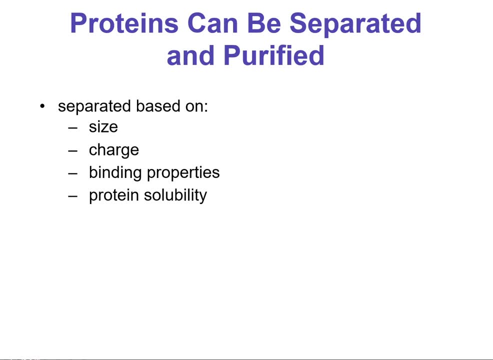 essential for the protein's function. Here's my favorite part working with proteins. So proteins can be separated and purified And we can use the different properties of our protein of interest to separate it away from everything else. You can separate based on size, charge. 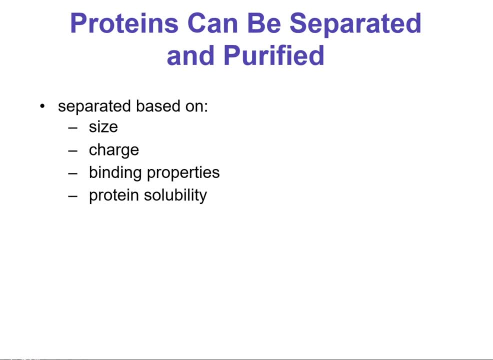 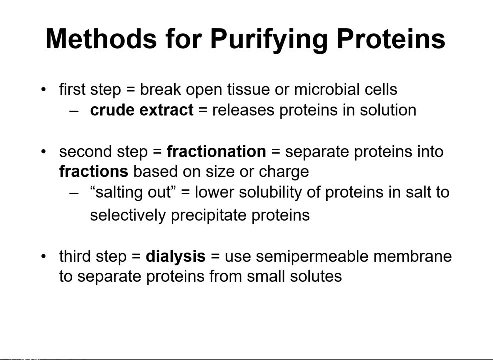 binding properties and solubility In general. when you're purifying a protein, the first thing you're going to do is take your protein source, whether it's a tissue or a microbial cell that you've overexpressed your protein of interest. 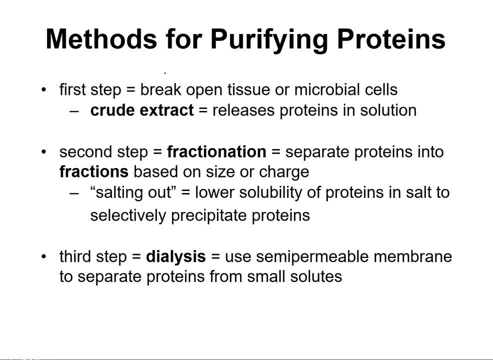 in and you're going to break it open. It's also called lysis. This gives you a crude extract. It's all the proteins from the cell or the tissue that you're purifying And you're going to break it open. 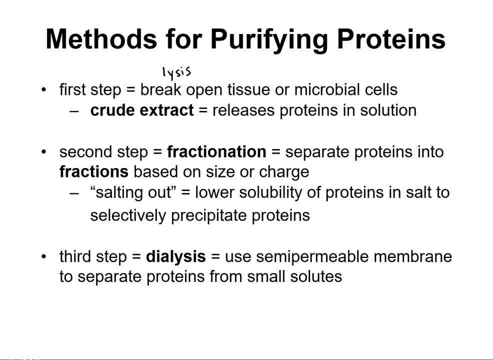 The second step is fractionation, And so you're separating proteins based on size or on charge- Lots of different things that you can do there. You can salt out a protein where you can exploit the differences in solubility. Lots of ways that you can fractionate, and we'll talk about that in just a second. 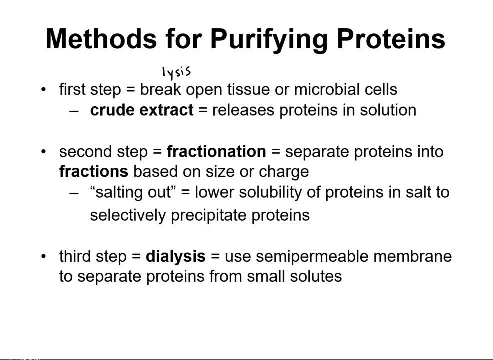 The first step is to sort out the protein, And you can sort out proteins based on size or charge. Here's my favorite part: working with proteins: You can separate from tissue of interest a second. then the third step is dialysis, and that will take away all the salt and 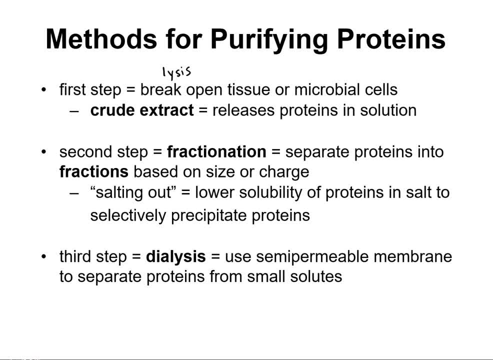 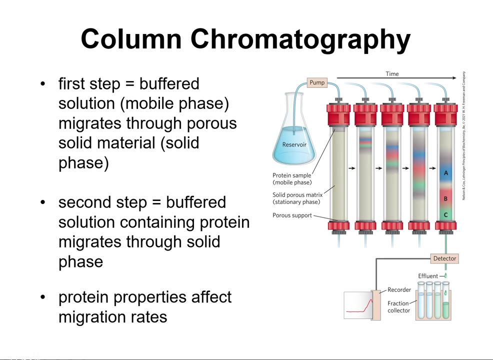 other things that you don't want with your pure protein, away from your protein of interest. when you're storing proteins, when you're using proteins high salt, metal contaminants- all sorts of things can interfere with the function of your protein. so column chromatography is something that, if you are into proteins, 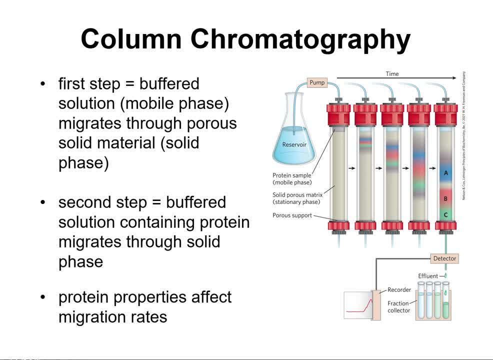 or enzymes you may end up doing a lot of as a graduate student or if you choose to do research like an MD PhD program, if you're interested in pre-med. so this is definitely something that, if you're interested in it, you could spend a lifetime learning about this. so the first step with any column chromatography is you. 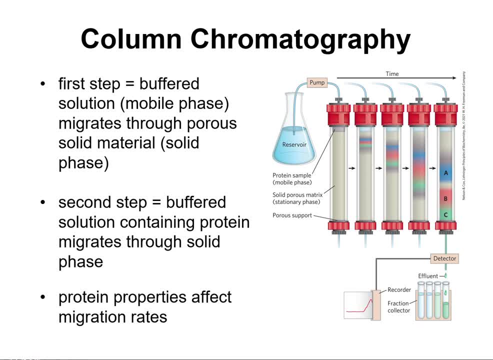 have a buffered solution, which is called your mobile phase, that migrates through some kind of porous solid material and that's called the solid phase, and that porous solid material is going. it can have different properties that you're going to exploit, so it could be charged and it could have. 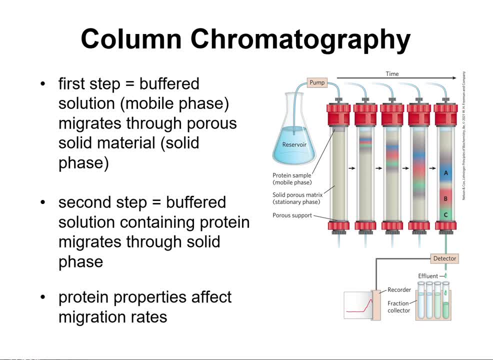 some kind of a ligand that your protein is attracted to you and will bind to. so that mobile phase is the buffer that has you know it's going to make your, your solid phase, ready to receive your protein. so the next step is to take a buffer solution that has your protein and migrate that through the solid phase. 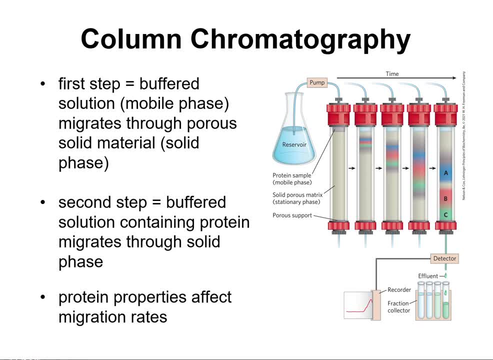 and hopefully your protein will interact with the resin, or maybe it's the only thing that doesn't interact with the resin, that's, you know. also possibility and the properties of your protein are going to affect the migration as the proteins migrate through the column. you can collect them using a fraction collector and you can detect using usually using. 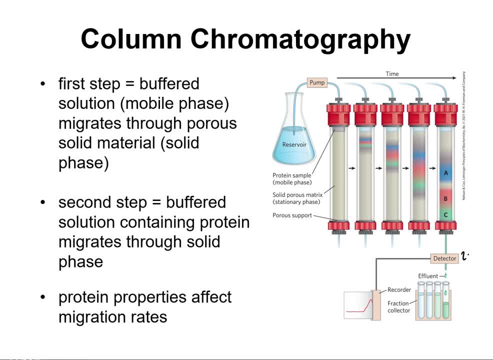 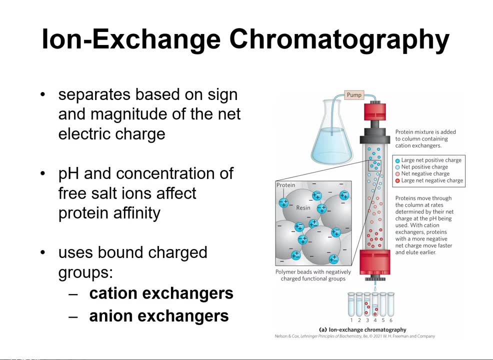 UV. these, so 280 nanometer light which we see, by the way, is size and thin, and a factor of two which gives us a lot, said will detect those aromatic R groups of amino acids. you can use that to detect protein. so different types of chromatography, ion exchange, very popular. 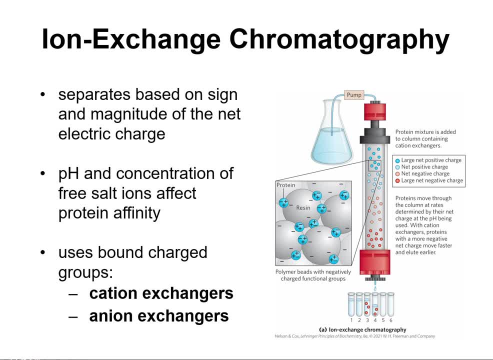 it separates based on the sign and magnitude of the net electric charge of your protein. so remember, proteins are made of amino acids and those amino acids all have, you know, ionizable components. some of them have our chains that are ionizable. all of that together gives the protein itself a charge at 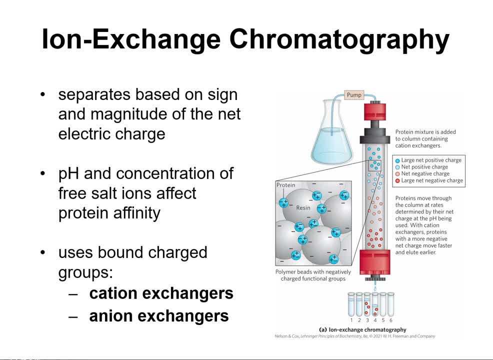 different pH is, so it may be positively charged, negatively charged or neutral, and you can calculate that and then exploit that to be able to isolate your protein away from everything else. so pH and the concentration of salt will affect your proteins ability to bind to an ion exchange column. you can use cation exchangers or anion exchangers. 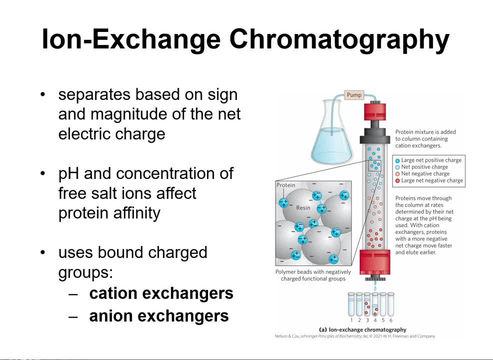 cation exchangers, which is what's pictured here. you're going to have negatively charged resin and you're going to have positively charged protein that interacts with that resin. with an ion exchangers, you've got positively charged resin and negatively charged protein, omega-3 3 and again you can achieve that by changing the pH or the salt. 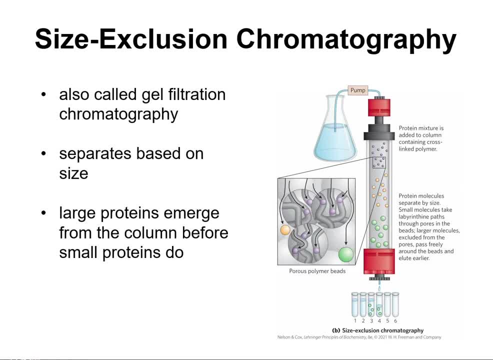 concentration. there's also size exclusion. size exclusion does exactly that. it will separate basically from groups of pollutants, which isn't really eye möglich, so you just have to keep that in mind. or Kanal Sports are bit different, but if you don't use any, an pane, so you just 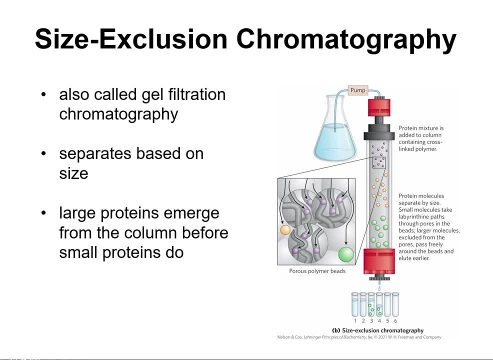 this is the soil hours method which is available on the network website is in org Trainer's exerc escolera. on size, You'll also see it called gel filtration. Same thing: The large proteins are going to emerge first from the column and then smaller and smaller and smaller. The large proteins can't. 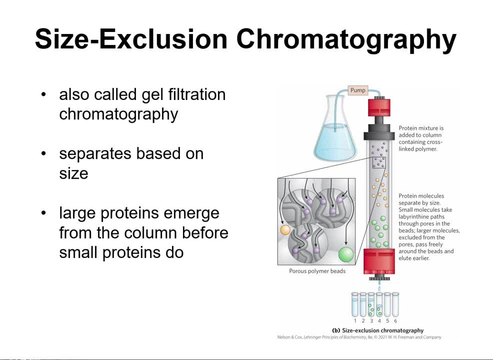 really interact with the resin, so they pretty much just go straight through. They kind of take the bypass the express lane and go straight through. But the smaller proteins are small enough to interact with the matrix and so they're interacting with the components of your solid. 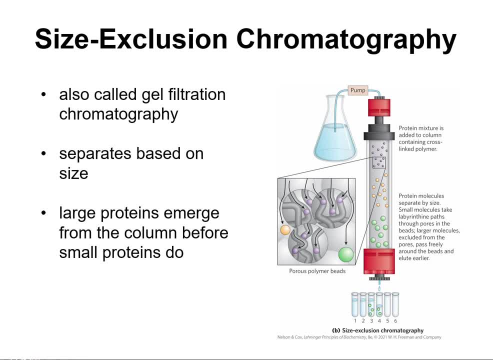 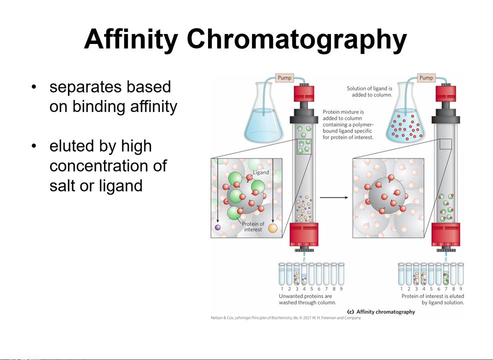 phase and it takes them time to travel through. So the smaller the protein is, the longer it takes to travel. Large proteins elute first, and then smaller, smaller, smaller. Then you can have affinity chromatography and this is based on binding affinity, So some proteins interact with a ligand. 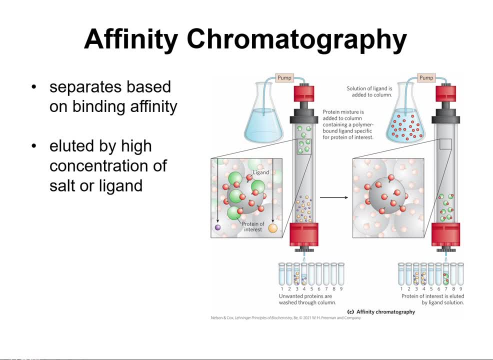 and that's just a small molecule that it will bind to and it'll bind really strongly. You can exploit that and have your protein bind to that ligand And everything else will just keep on going about its business. You can also use protein tags, So you 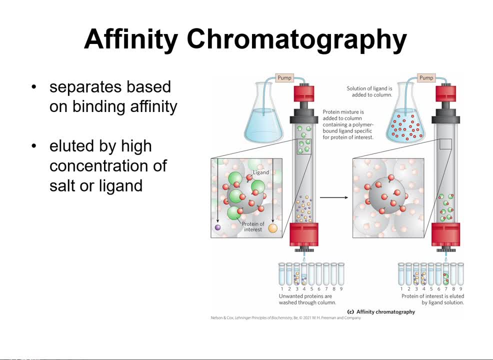 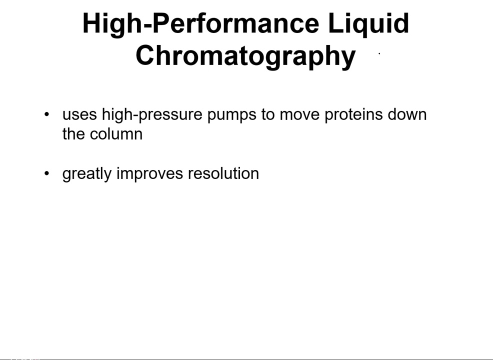 can express proteins with a tag that it wouldn't normally have out in nature, and that tag can be attracted to some kind of ligand on a column, So that is also a great way to purify a protein. You can use HPLC- high-performance liquid chromatography- and that uses high-pressure pumps to move. 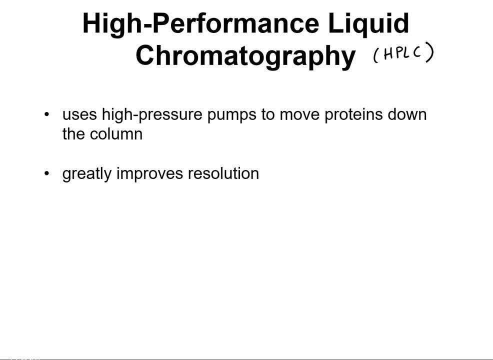 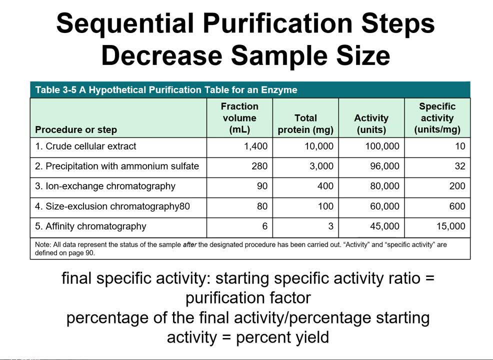 proteins down the column and that will improve your resolution as well. So here we're just looking at the different steps in the procedure and how pure your sample is. So in the beginning you've got this crude cellular extract And in that extract you have a ton of protein, right? 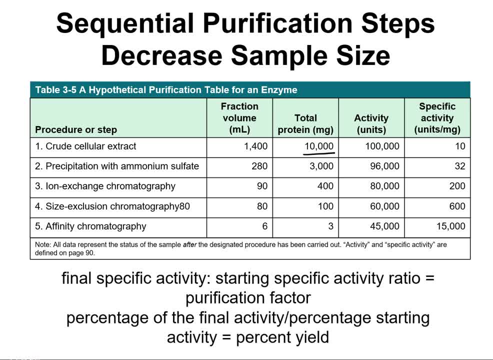 Lots of protein here. But in terms of your specific activity- whatever reaction your protein catalyzes- pretty small because that activity is diluted over a pretty large volume As you continue to purify and fractionate. your specific activity increases because you're removing more and more. 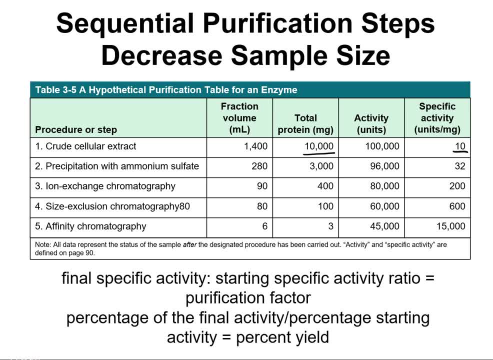 contaminants. Until at the end, your last step, you've got a very small volume, But that small volume is all your protein, So your specific activity very high. And that's how you purify and fractionate. And that's the goal: To have a small volume, lots of specific activity from your protein, which means that you've got a lot of your protein. 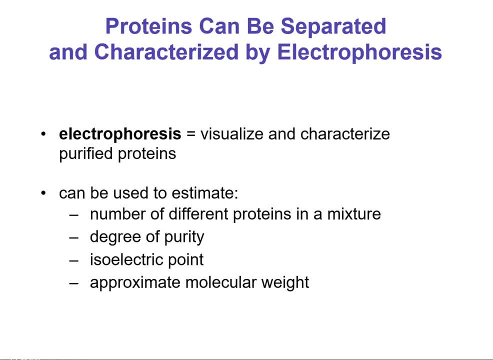 Now we can't just blindly do a purification process and say, okay, we're done, There's protein in these tubes, I dialyze them and I'm ready to go to town. You need to use some diagnostic tools to actually make sure that you have the protein you think you have. 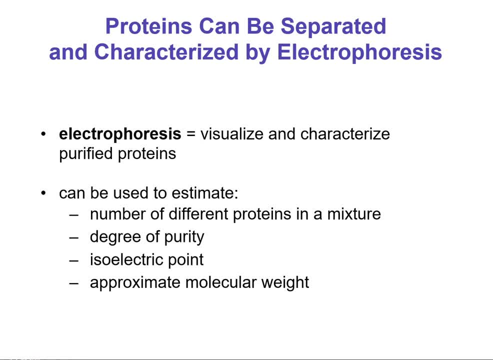 One of the tests that you can do is looking at the size of the protein using electrophoresis. This is a technique that you can use to visualize and characterize purified proteins, So you can estimate the number of different proteins in a mixture Which is kind of related to that degree of purity, which is the next point. 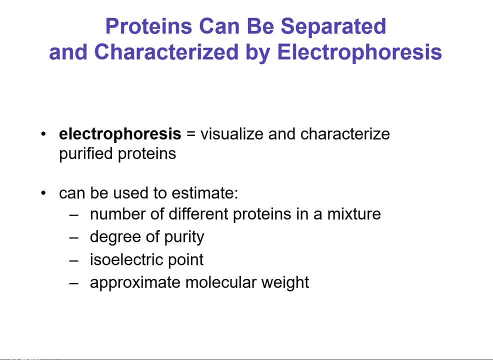 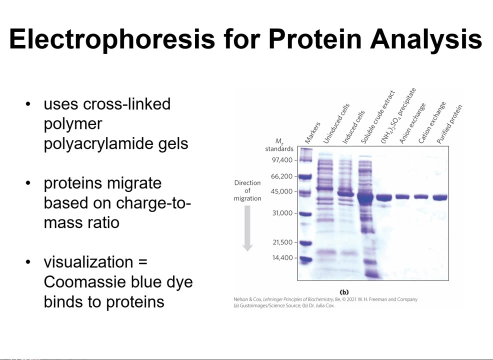 You can identify the isoelectric point And you can also approximate the molar weight or molecular weight of your protein. So you're going to take your protein sample and use an electric field to migrate those proteins across a polyacrylamide gel. 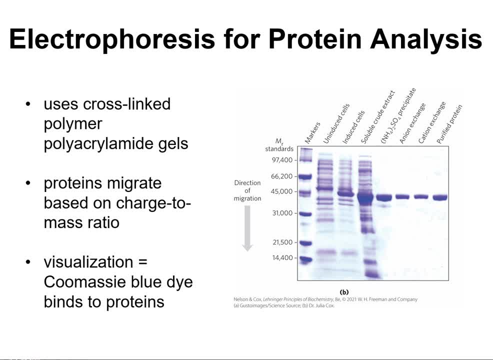 And you're going to take your protein sample and use an electric field to migrate those proteins across a polyacrylamide gel. The proteins migrate based on a charge-to-mass ratio And they're visualized using Kumasi Blue dye. There are other ways that you can stain, but Kumasi Blue is pretty standard and it's the easiest. 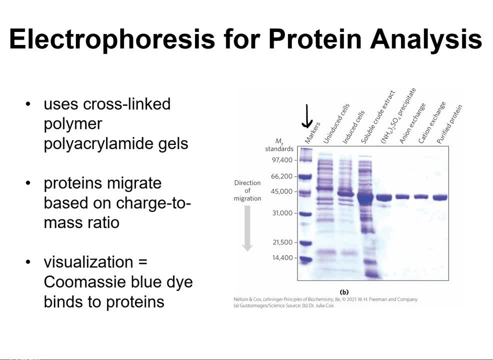 Notice that in this first lane there are markers. These are molecular weight markers And that is just a standard that you can purchase that has specific amounts of proteins with known molecular weights And you can compare how your protein runs to the molecular marker to get an idea of what your molecular weight is. 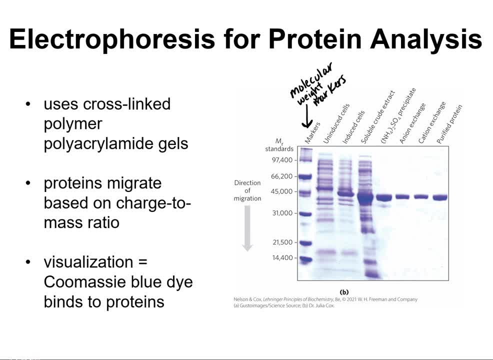 The next thing you want to do is to compare your protein to the molecular marker. The next lane has uninduced cells And we're going to talk more about this in class. But if you're overexpressing a protein in bacteria or some other cells, 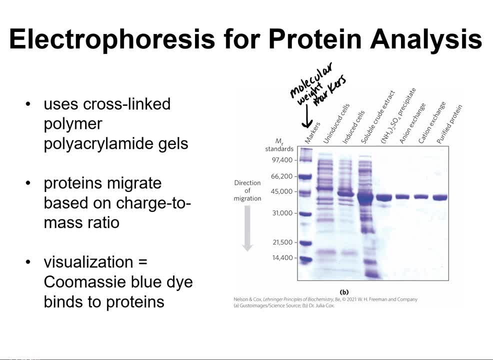 you can crack open those cells before you start overexpression and take a look at what your protein composition is, And then you can induce and all of a sudden you see this band of protein appear. That is very likely your protein of interest. 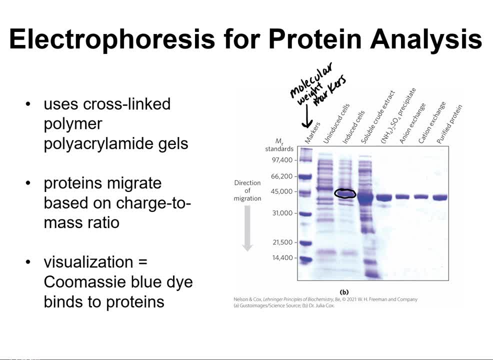 Then you lyse the cells and you have your crude extract. Again, you see this large band here. You do an ammonium sulfate precipitation, Anionic exchange and all these other. whatever other things you're going to do, You can do that in a certain way. 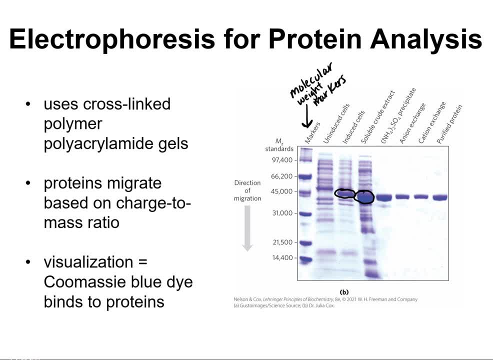 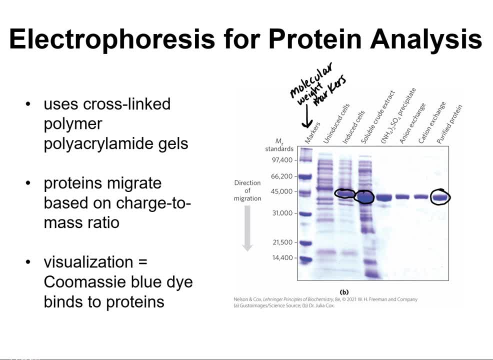 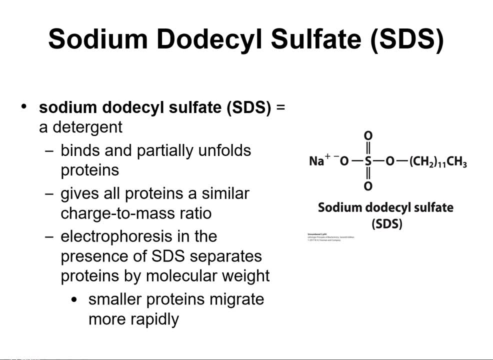 beautiful looking band at the end and hopefully it's what you want. when you're running a protein gel, you are very likely going to be using sodium dodecyl sulfate or SDS. it is a detergent. it binds to proteins and it partially unfolds them so that you're not running. you're not running a native gel, that. 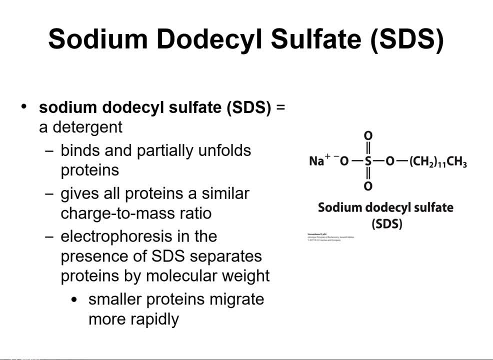 you're running a denatured gel. that means that the proteins are kind of relaxed and open and you're going to have a similar charge to mass ratio for all your proteins, so that the only difference is: well, this protein is a denatured gel, so that the only difference is: well, this protein is. 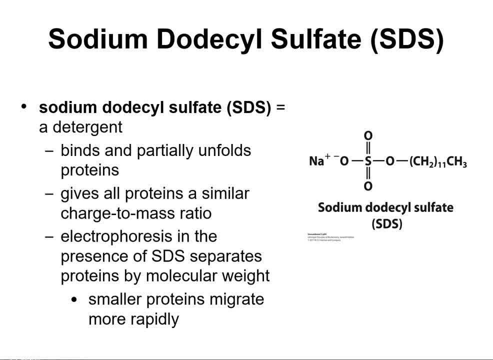 protein is bigger than another protein, so it's going to move more slowly than the smaller proteins. so SDS helps to separate proteins by their molecular weight, because we're not taking into account the differences in the protein size and shape. there are ways that you can run what's called a native gel and 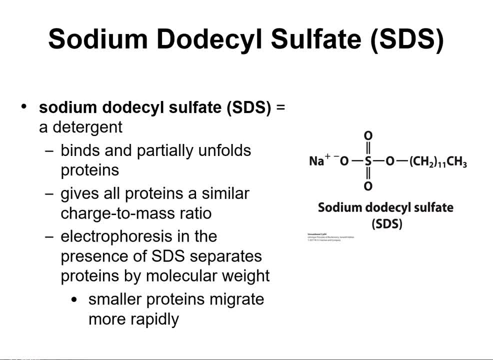 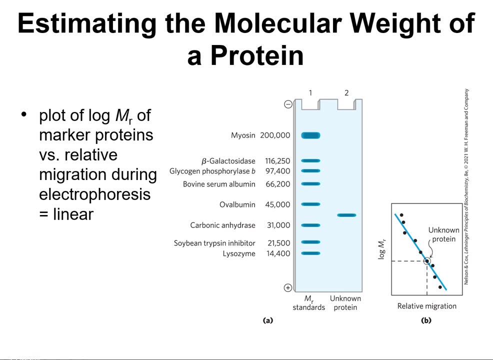 that takes the protein as it is and let's run through a gel, but oftentimes that's for a specific reason and you're not usually using that when you're doing protein expression purification. if you want to estimate the molecular weight of a protein, you have to have some kind of molecular weight marker proteins and 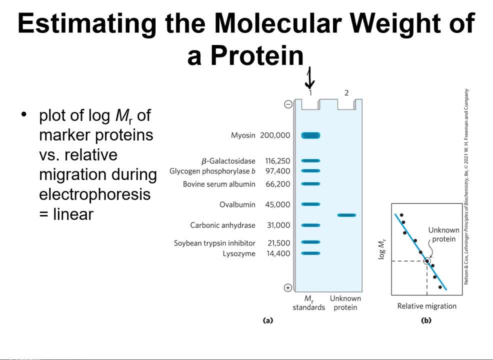 that's what's again in this first link. usually this is something that you purchase and you receive, you know, some literature along with your purchase that tells you what the proteins are and their size and daltons, if you plot this, the distance of the, their migration on the gel. 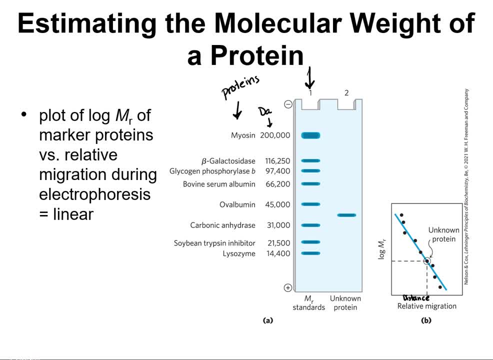 versus the log of their molecular weight. then you will get a standard curve and you can take a distance measurement of where your protein runs and then you can kind of have an idea of what the log of that molecular weight is and then from there you can figure out the molecular weight of your protein. it's not perfect, but 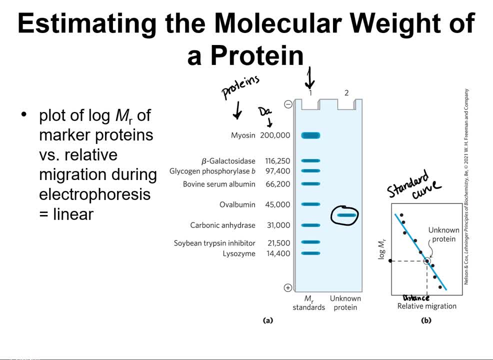 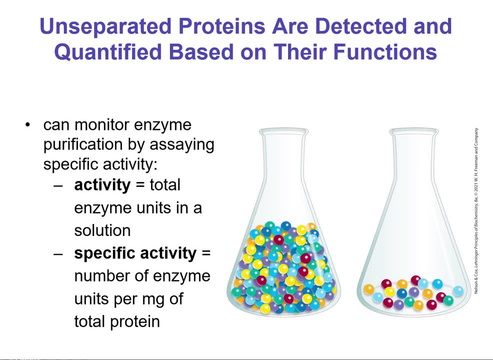 it's definitely. you know it gets you in the ballpark, so you can just came out with such an idea and then you can do some computations to make sure it's very accurate and you can figure out the information right after that. and if you want to do more, you can probably do that, but you can. 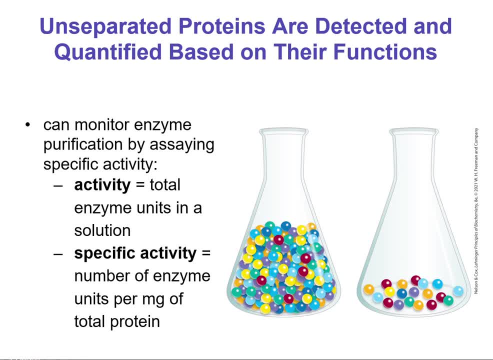 either go back to your reference notes or you can take that and you can do that, and then you can make sure that that's the right answer, and then you can see that those are the exact same elements that are present as the same elements in a particular cell. to be able to predict how this is going to be, 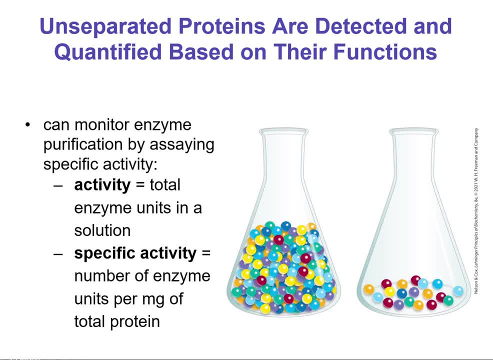 enzyme and that that activity is increasing over time. so activity is the total enzyme units in a solution. specific activity takes into account the amount of enzyme activity per milligram of total protein. so that is the number that was in the chart a few slides ago. that takes into account. okay, we've got. 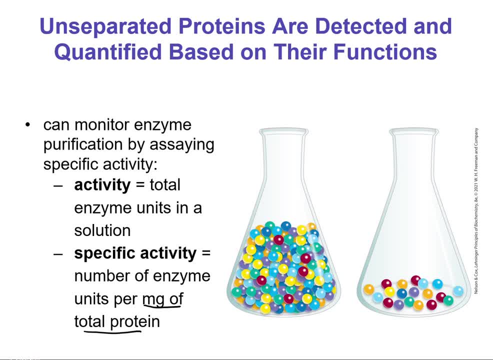 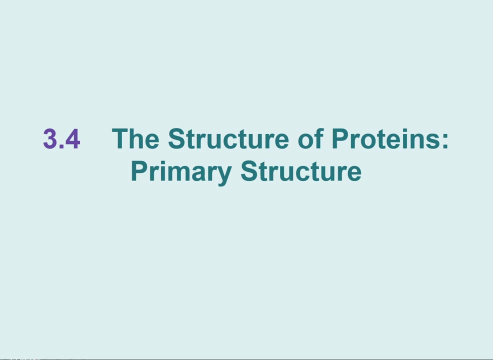 all this protein, we've got this much activity. as you purify, the number of milligrams of protein, total protein, goes down, which means your specific activity should increase over time. so over the course of purification it should increase. now we're moving on to the structure of proteins. there's different levels of 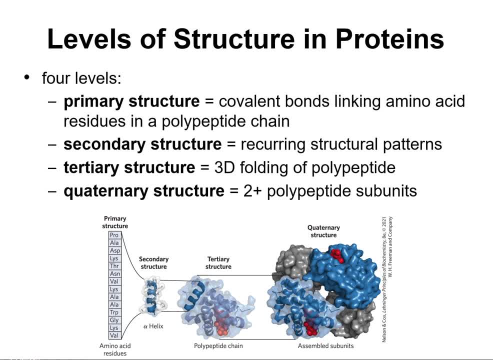 structure. there's four levels: primary, structural and secondary structural. there's four levels: primary, structural. there's four levels. primary structural. there's four levels: primary structural, which is just the amino acid sequence. the secondary structure is looking at recurring structural patterns: alpha helices, beta sheets. those are secondary structure. tertiary structure, where the 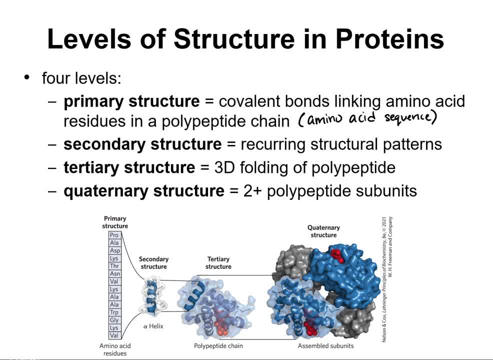 we're talking about the 3d shape of the protein, and quaternary structure is when we're looking at more than one subunit. so if you've got multiple subunits that come together to form some kind of complex, that would be quaternary. 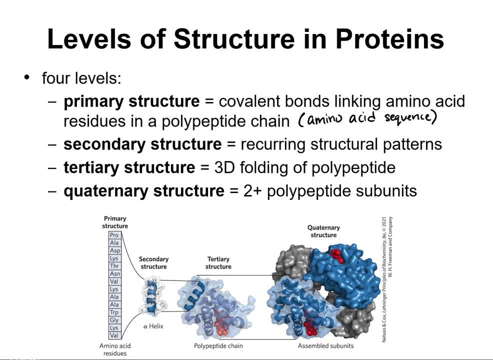 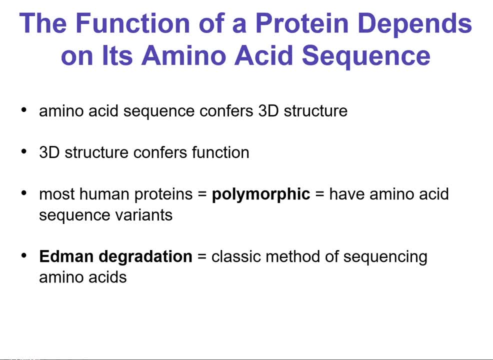 structure. the amino acid sequence informs the 3d structure and that structure is important for us for specific functions. so if you know something about the function of the protein, that you may be able to guess what its structure is. if you know about other proteins with similar functions and the reverse, 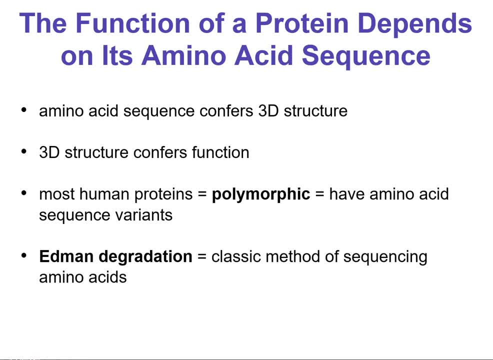 is true as well. if you find some unknown protein and you can figure out its structure, then you may be able to guess what its function is. most human proteins are polymorphic and that means that they have variations in their amino acid sequence. but remember, with the amino acids we have different. 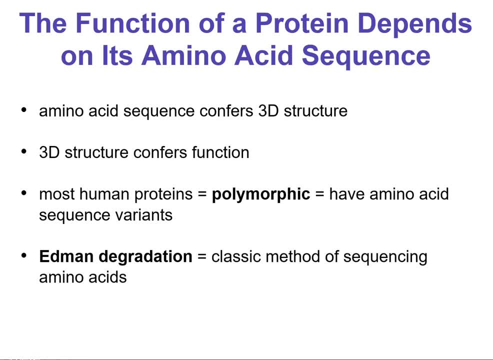 proteins that are polymorphic and that means that they have different classes of amino acids and you may be able to substitute one amino acid for another and still maintain the overall characteristics, so you can have something that's aromatic. we've got a few choices for that. you want something? 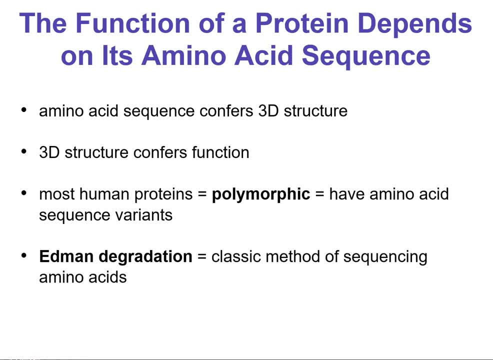 nonpolar and aliphatic, there's a few choices for that. charged, there's several choices for that. so, doing those kinds of swaps, it could be a net zero change in terms of the structure and function of the protein. because proteins are so important to life, in order to study them, we ought to be able to take them apart. 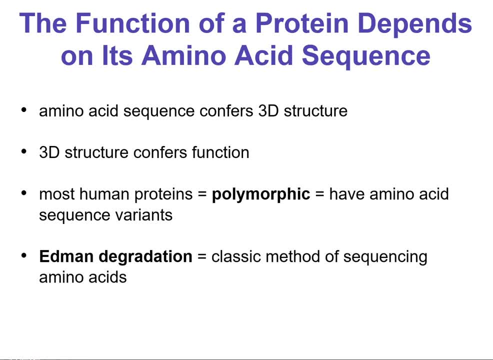 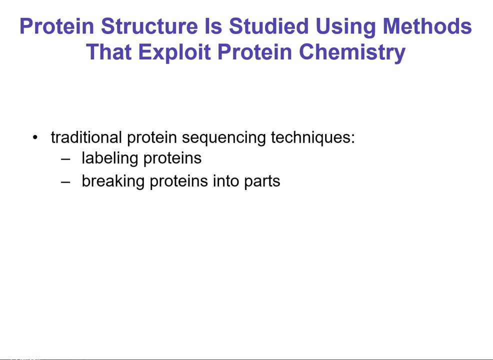 and Edmund. degradation is a classic method of sequencing amino acids. other techniques for sequencing amino acids and big polypeptides have been developed based on this method. Traditionally, when you're trying to figure out the sequence of a protein, you've got two options: you can label the protein and figure it out. you can break. 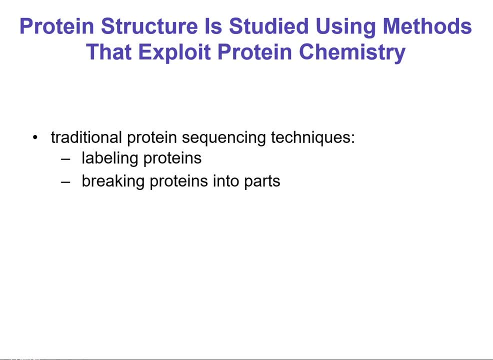 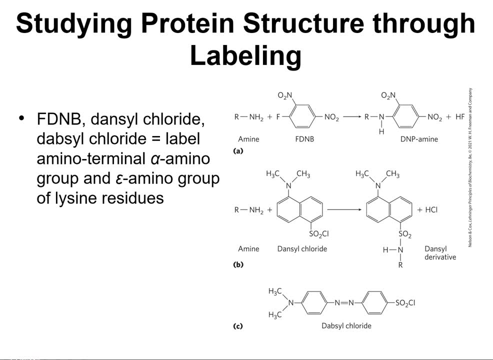 the protein apart. figure it out if you're going to use labeling. there are lots of different chemicals that will label the amino terminal amino group. so remember the first amino acid has that free amino group and that is available to do chemistry so you can modify with all kinds of different. 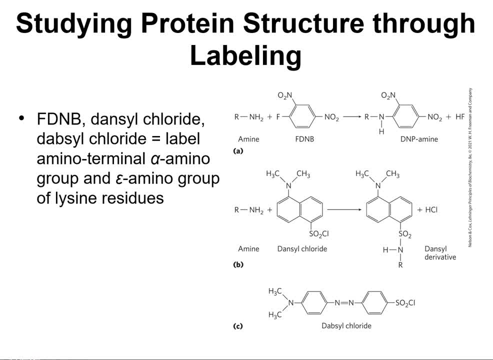 chemicals to label that group and from there you can do a whole host of things to isolate one peptide at a time, and when it comes to Edmund degradation, you're going to first label and that is at higher pH. then you can cleave that labeled protein or that labeled amino acid at low pH and 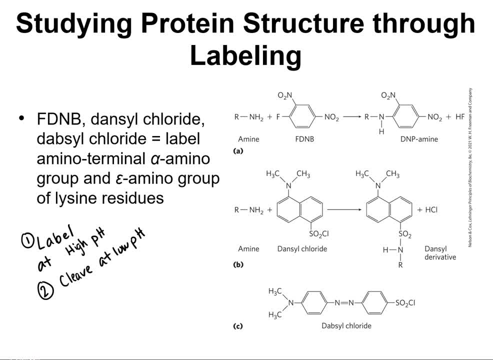 taking advantage of the difference in pH means that you can have labeling complete, hundred-percent and then change the pH and have cleaving 100% and then from there you can identify the free amino acid and then start again: label cleave, identify the free amino acid and all these labeling. 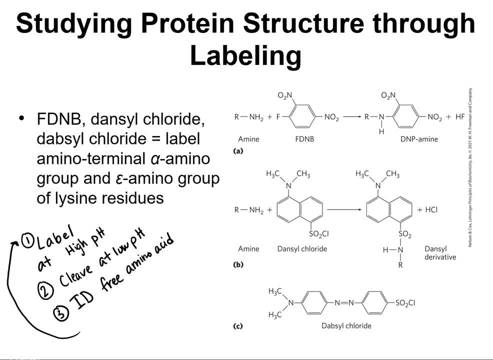 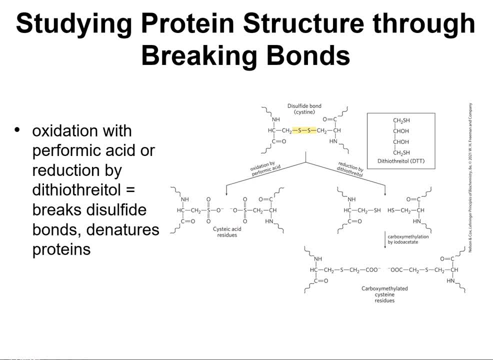 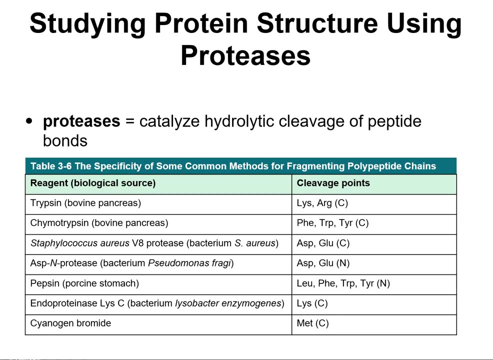 techniques are based on that kind of a premise. you can also study protein structure by breaking bonds, so you can break di sulfide bonds and then see what happens. you can do nature proteins. we not really going to focus on that too much, though. one great way to study protein structure is using proteases. proteases are enzymes. 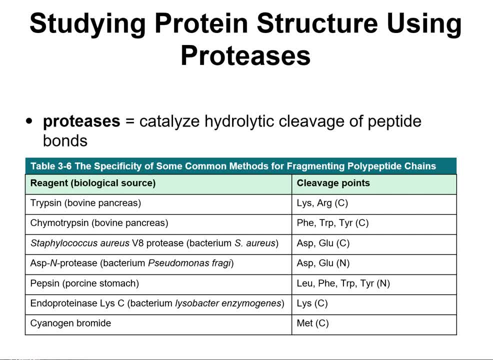 that like, for example, to form a sauteic protein from willing to upload 케아�asedde, catalytically hydrolyzed peptide bonds far more efficient than chemical means. there's a whole host of different proteases. you don't need to know any of. 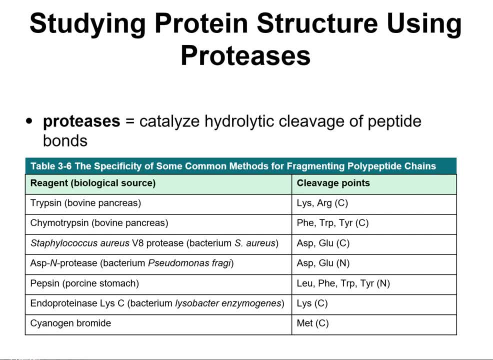 them specifically. but you should know that different proteases have different cleavage points so they recognize certain sequences of amino acids and they will reliably cleave proteins in those areas in a certain way and you can take that information and you can say: digest a protein with two or three or 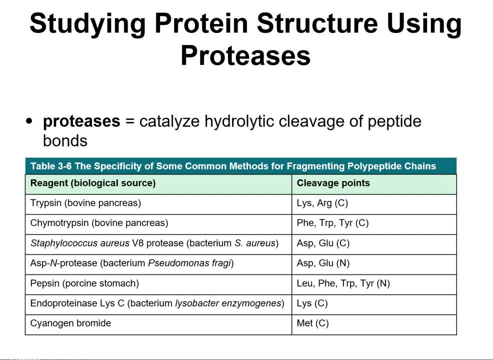 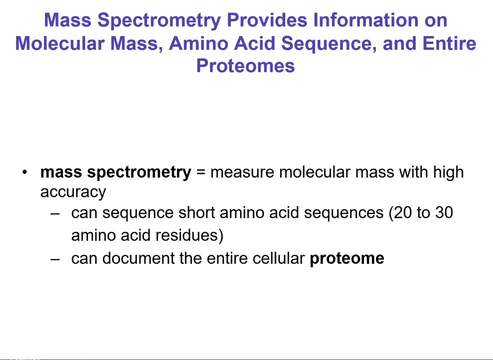 five different proteases and use the overlapping sequences to help figure out the entire protein structure. you can couple that with mass spectrometry so you can digest a protein and then use mass spectrometry, which helps you to measure molecular mass with really high accuracy. so you can sequence and you can actually. 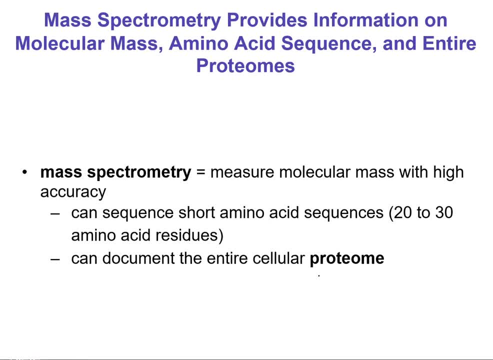 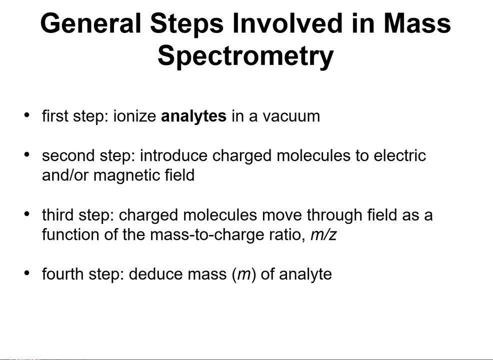 look at the entire proteome, which is all the proteins that are in one protein, and you can adjust these to theлекrast and you can create a different protein structure to help you to know what it's like and how to do it better. and I would love to hear from you guys in the comments in the 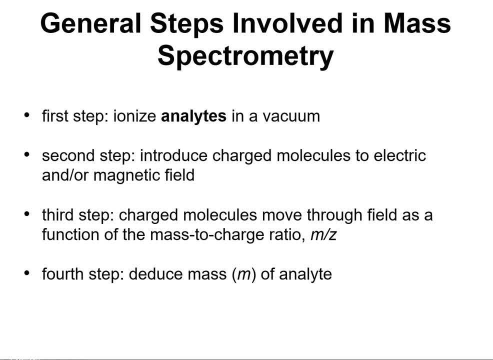 comments and I will see you all in the next tutorial. we're just going to talk about the general steps involved in mass spectrometry. mass spec is something that you could again spend a lifetime on: very interesting, very complex, a lot of math. believe it or not, these machines are like modern marvels in my mind and very powerful machines which are like modern marvels in my mind and very powerful machines which are very powerful and very powerful machines which are 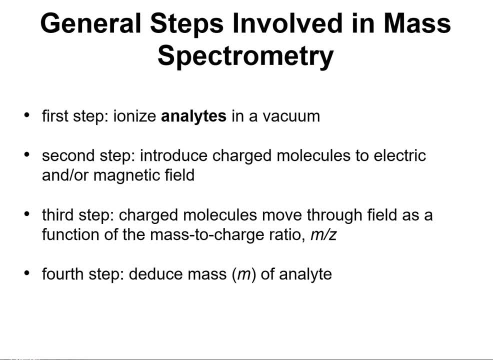 powerful tool. If you're interested in doing any kind of research, especially like metabolic research where you're looking at a lot of different metabolites, mass spectrometry is something you'll definitely want to learn about. The first step for mass spec is to ionize the 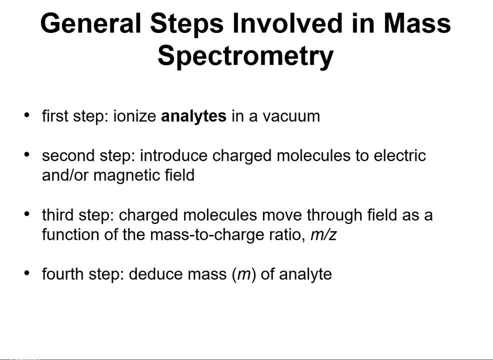 analytes in a vacuum. What that means is you're going to take your peptide pieces- those are the analytes- and you're going to give them a charge. Then you're going to introduce those charged molecules to an electric field or potentially a magnetic field. There's lots of different mass. 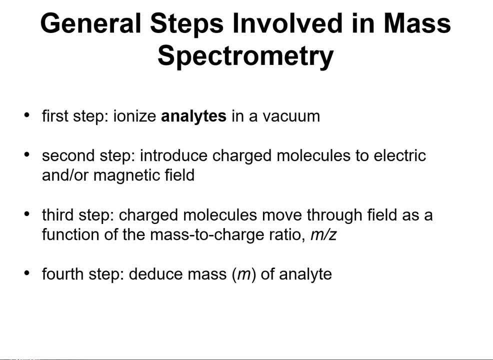 spec. There's lots of different ways to ionize and then introduce to a field. There's different types of mass spectrometry, so it really depends. Then those charged molecules move through the field as a function of their mass to charge ratio or the m over z. 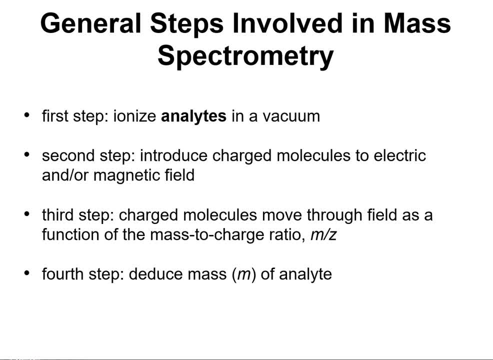 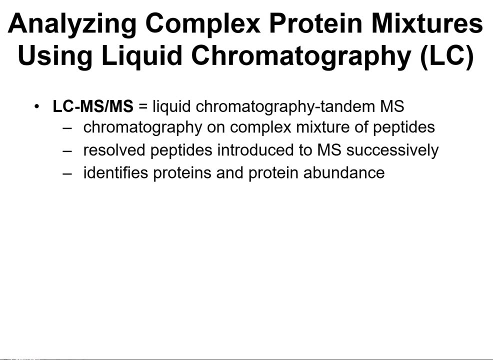 Then, after that, you can deduce the mass of your analyte. Again, we're not going to go into detail about how to do all those things. We will talk about combining liquid chromatography, which is what we talked about, with all the affinity columns and the ion exchange. 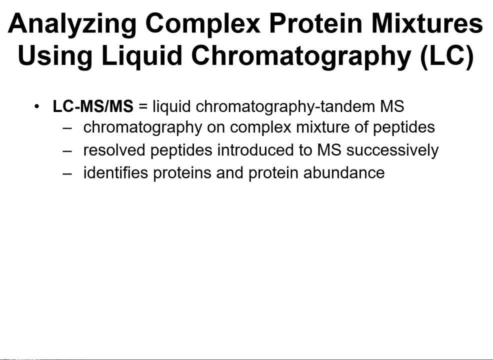 and things like that. You can use liquid chromatography along with mass spectrometry. You can link up different types of mass spectrometry. You can do what's called LC tandem MS. You can have mixtures of peptides and that's how we get to looking at the whole proteome. 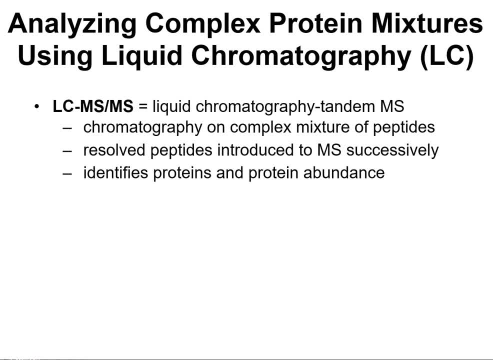 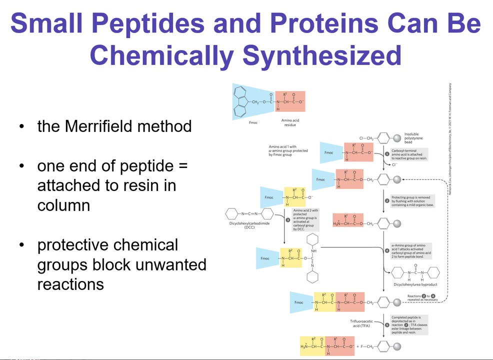 Resolve those peptides that you first used chromatography to separate, Then look at mass spec. Then you can identify proteins and protein abundance. Very cool stuff. Not going to bore you with it, but if you're interested let me know. We talked a lot about figuring out the sequence of a protein. 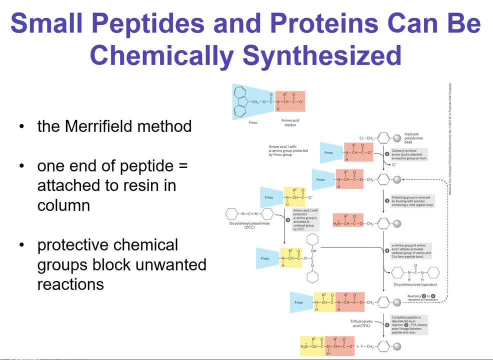 You can actually make proteins too. If you wanted to make a small peptide or a small protein, you can do that chemically. We're not going to talk specifically about the method, even though it is shown here on the right. We're just going to talk about a couple of the main points in terms of how you do this. 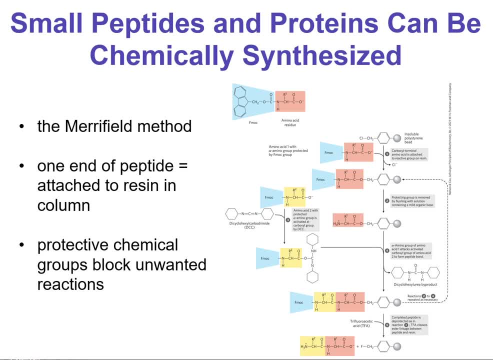 You have one end of your peptide that's attached to resin on a column And you protect the ground of your peptide. You protect the groups that you don't want to be chemically modified, Usually with Fmoc. Don't worry about what that is. 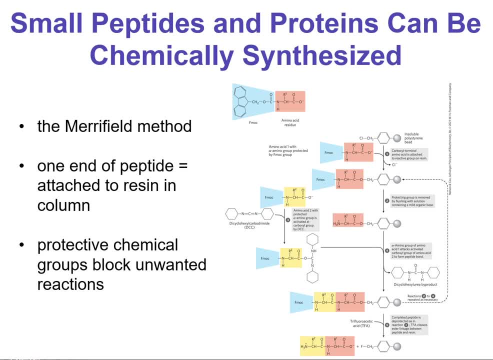 Just know that it's a protectant. You can use whatever chemistry you need to add on your next amino acid And then you block that. And then you continue over and over again until you have made your peptide or your protein Chemically. it's not exactly the most efficient. 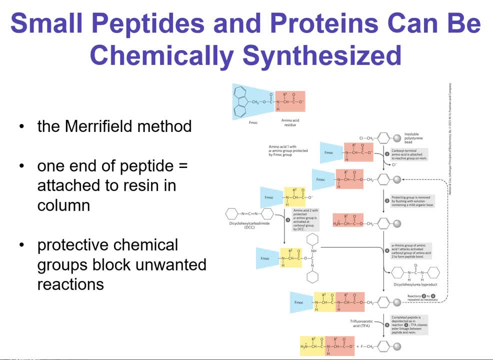 Enzymes are much better at this than we are in the lab, But if you need a small peptide or something for what you're doing in the lab, it can be an alternative to purchasing a peptide. There are actually automated machines that will do this for you. 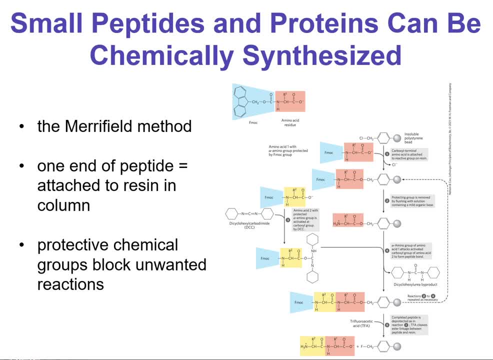 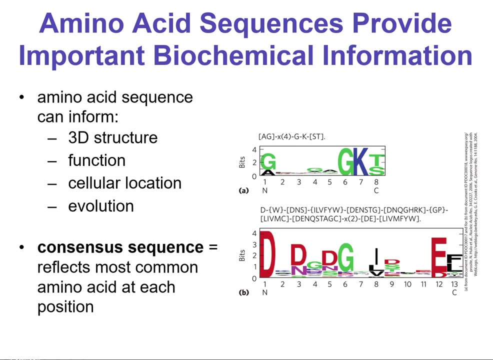 versus you having to do all of the steps yourself and be your own organic chemist. So that's all we're going to say here about synthesizing your own proteins chemically. So a couple more notes on amino acid sequence. The sequence of a protein can provide biochemical inhibitors. 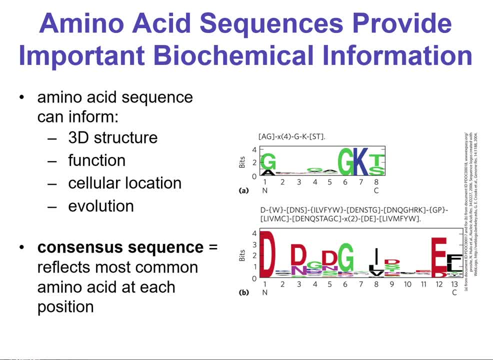 And biochemical information. We already talked about how it can inform the structure, So the tertiary structure and the function. But we can also get information about cellular location. So maybe there's a tag or a sequence at the beginning or the end of the protein. 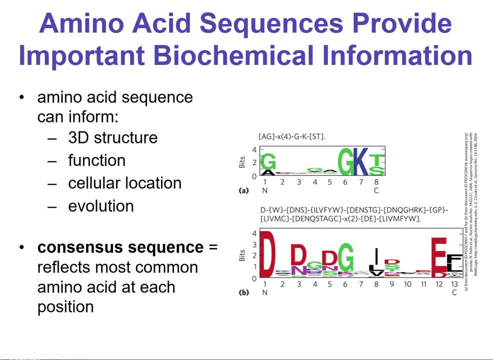 that all proteins with that tag are localized to the endoplasmic reticulum, Or there's some kind of prosthetic group that we know binds to this particular region And that prosthetic group maybe localizes it to the cellular membrane. 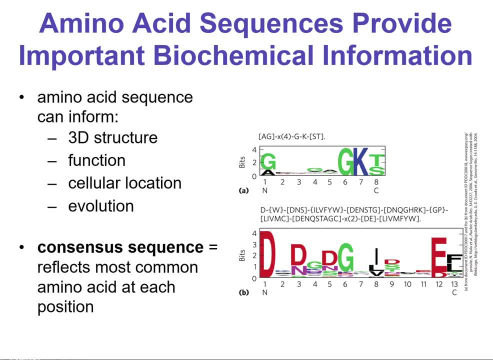 We can also look at evolution. So the really important residues in a protein or an enzyme are typically conserved. Even when you look at different species, you can look at: Oh, So these residues have not changed, These other ones are variable. 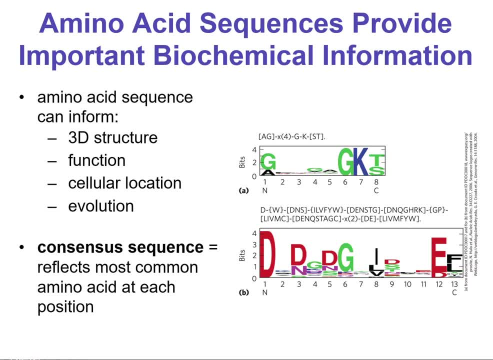 But at these points we typically see this amino acid residue here. So on the right, what we're looking at is kind of these conservation charts where the size of the letter indicates how well it's conserved, And then N to C- we're talking about the N terminus to the C terminus. 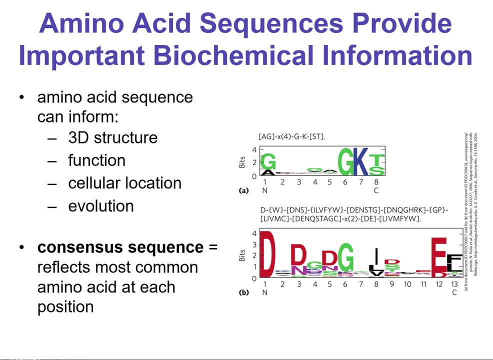 So really big letters conserved. So in B that D, which is aspartate, highly conserved. However there's some variation here. So there's some conservation, but not as much There's, It's variable there. 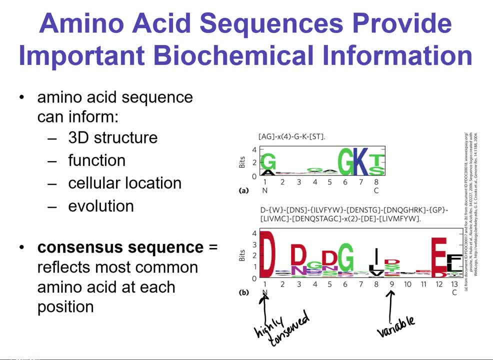 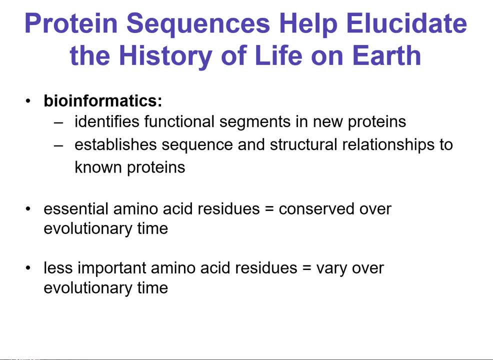 So this is also called a consensus sequence. You're looking at the most common amino acid at each of these positions. When you do that, you can actually help identify the functional segments of new proteins or unknown proteins And you can establish sequence and structural relationships. 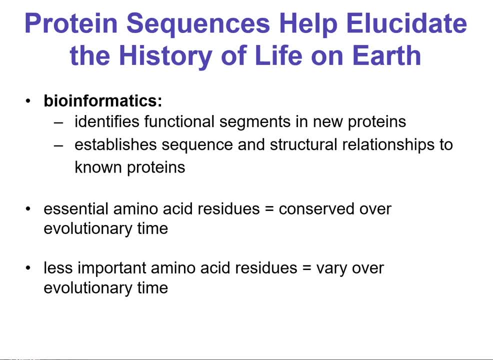 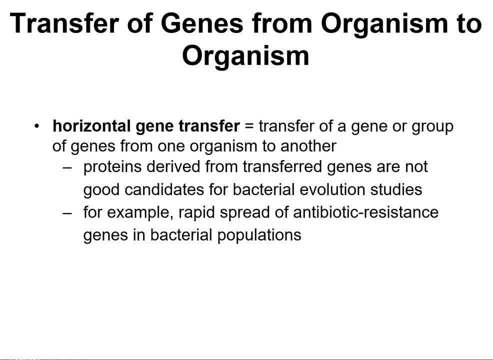 So if we know that- you know- this particular consensus sequence is associated with this type of enzyme activity, then we can start to establish different families and things of that nature. We can also identify what's called horizontal gene transfer, And that's when a gene 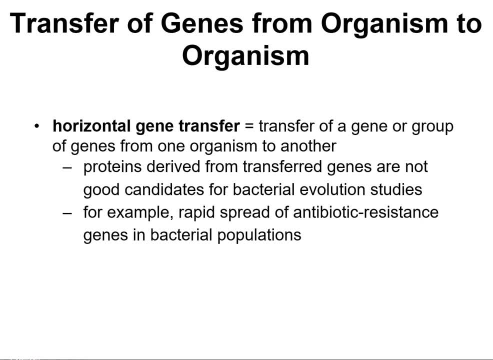 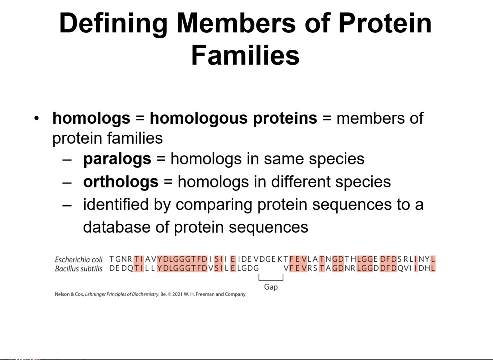 or a group of genes is transferred from one organism to another. When you're trying to look at evolution, these are probably not the genes that you want to look at And, like I said, you can use the evolution and look at these consensus sequences.